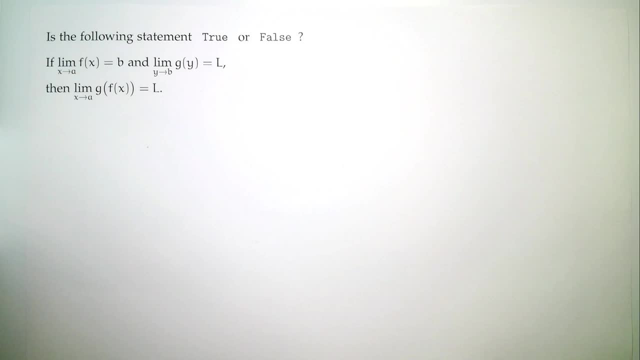 preference to one side as to whether it's true or false. Let's think about what the intuition says. So what's happening here? Well, if we think about this, this is sort of like what I like to call an onion problem, in that there are layers and that probably 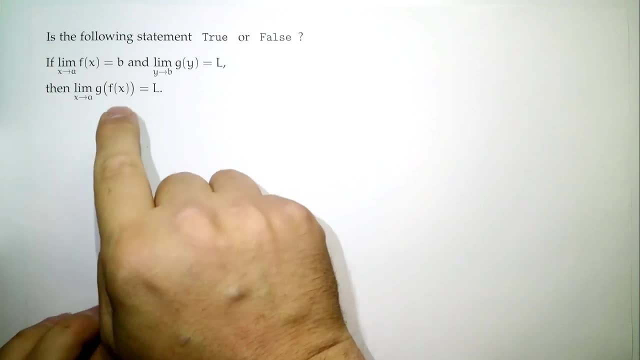 there will be a couple of tiers, But here we go. So let's think about from the inside: x is getting close to a, So the inside, I have f of x. So that says that the inside, our intuition, says the inside's getting. 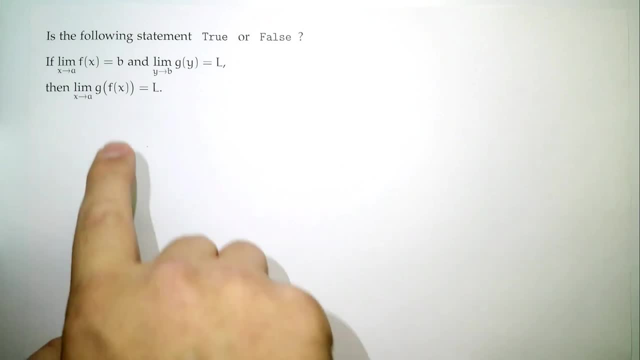 close to b. Okay, So when I say the inside, this whole expression, So when I'm plugging in to the function g, it's getting close to the value of b. And here I say if, when I'm plugging in to b, sorry, if when I'm plugging in to b, I'm plugging in to b, I'm plugging. 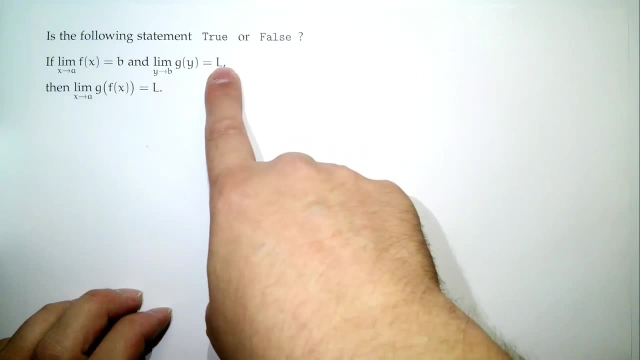 in to the function g gets close to b, then it should be near l or it goes to l. So when I'm plugging in to g, it's getting close to b, And so it seems reasonable that the answer should be that the limit is l. All right, So the intuition tells us the limit should. 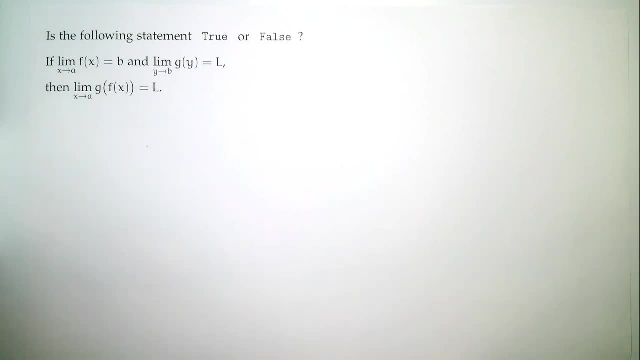 be l, So the answer is, of course, false. Now, if you take this question and you ask a grad student, they will tell you the answer is true. If you ask a faculty member, they will tell you the answer is true. Why is the? 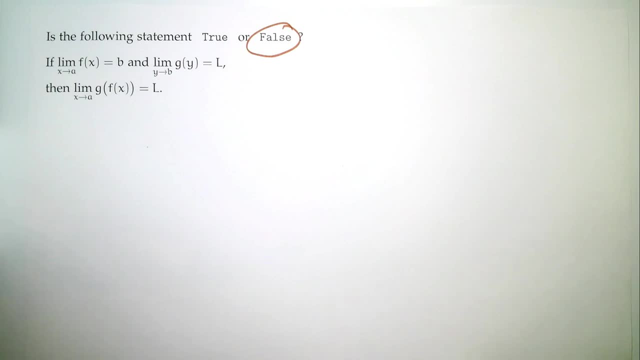 answer false. So, first off, what does it mean by false? When we say false in mathematics, we say there is some weird situation where the statement doesn't hold. So mathematicians have a really high standard for being true. It's a great way to get off of jury duty. You know the. 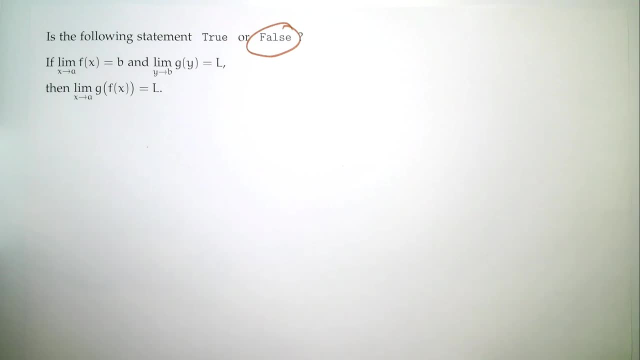 judge asks: well, what do you consider true? Well, I'm a mathematician. OK, that's it. Thank you, You don't need to be here anymore. So what's wrong with our intuition? Well, let me try to convince you that. first off, there is some case where the answer turns. 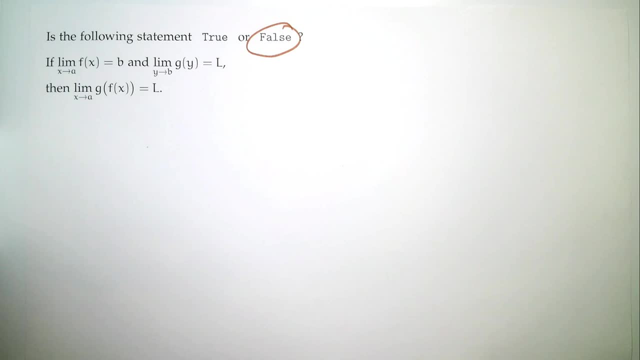 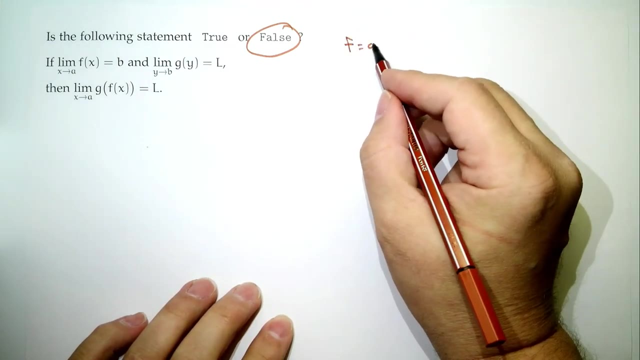 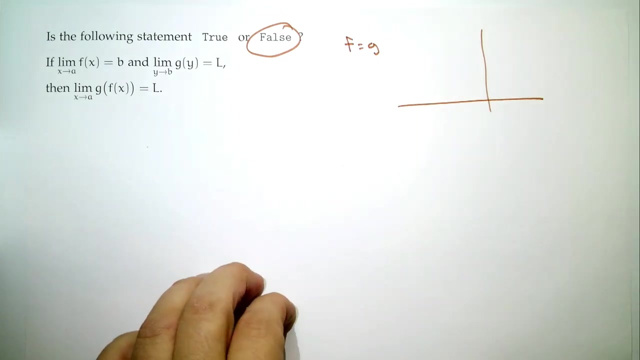 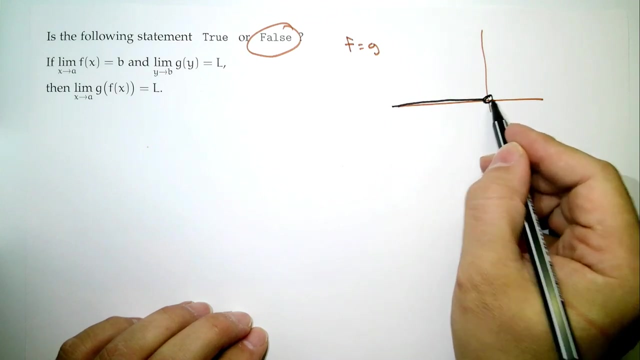 out that the limit is not what it should be. So I'm going to do a really simple example. I'm going to let our function f and g be the same function And I'm going to graph it And it's the following function: So here's my axes, And it's going to be 0, except at the value of 0, in which 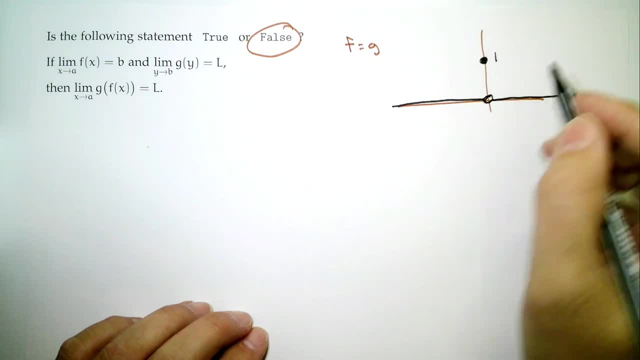 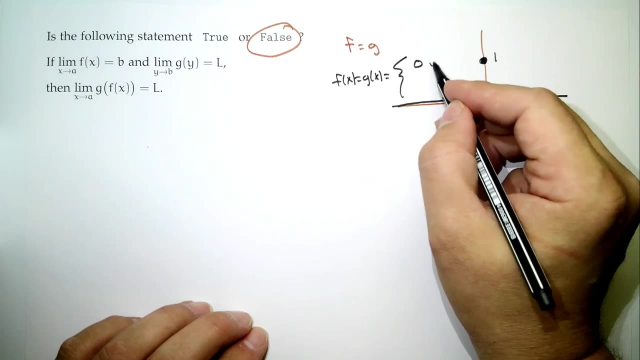 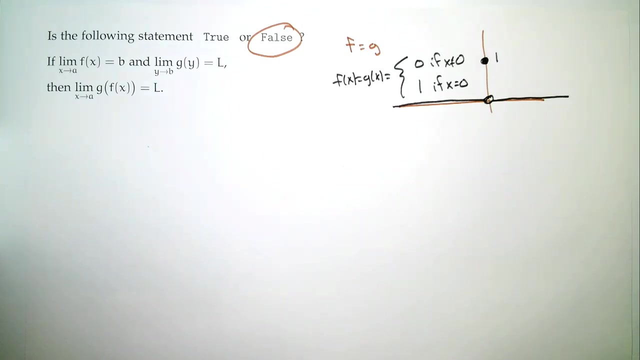 case, it's going to be 1.. So there's the function. So, in particular, f of x equals g of x equals 0.. x is not 0, and 1 if x does, equal 0. And now I'm going to let a equal b equal 0. So I have. 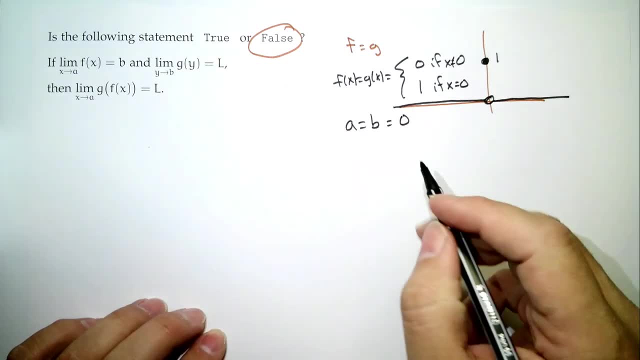 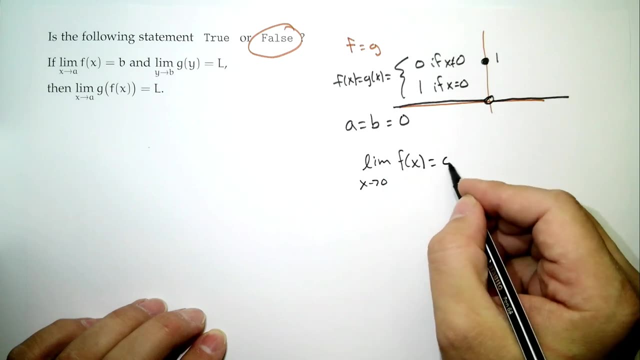 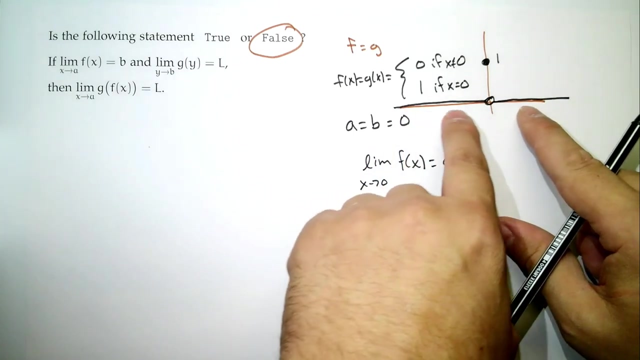 to check. does this statement hold? does that statement hold? So does the limit as x approaches 0 of f of x equal 0?? Well, we follow the picture in and the answer is yes, because as I go in from both sides, I'm still 0. So that's a true statement. So now we go to our next. 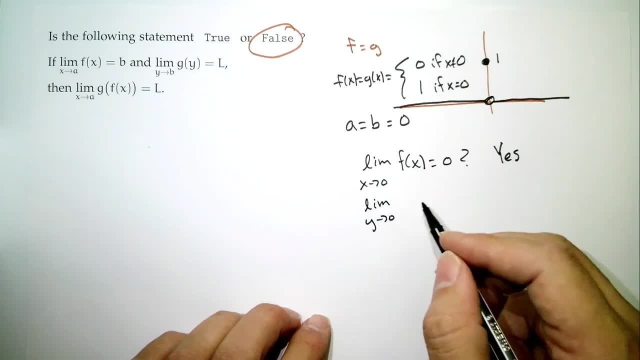 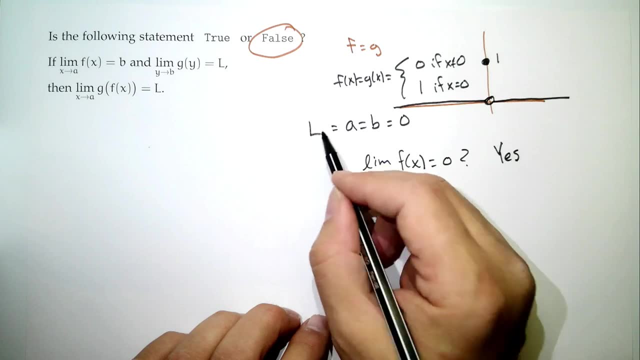 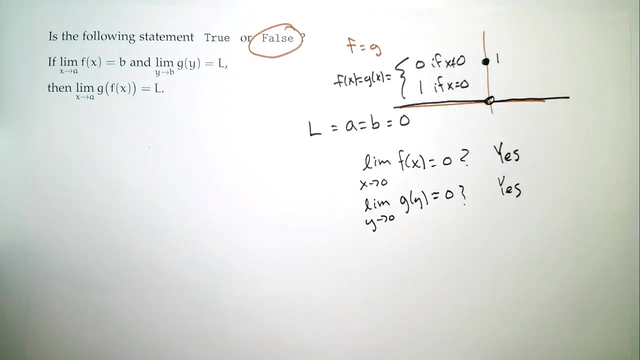 statement: Does the limit as y approaches 0, of g of y equal 0?? So I guess I should have said what l is. So I'm going to let a equals b equals l, and the answer is still yes, because it's the exact same function. I'm approaching the same point. all I've done is switch the. 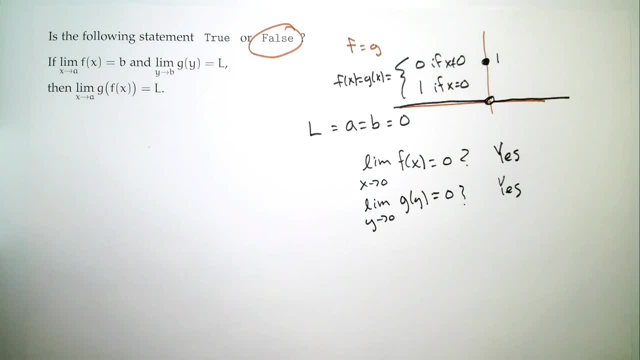 variable names. Okay, so so far both of these assumptions are true. Now let's figure out the following: What does the function g of f of x look like? Well, there's two possibilities. Suppose for a second that x is not 0.. So if x is not 0,? 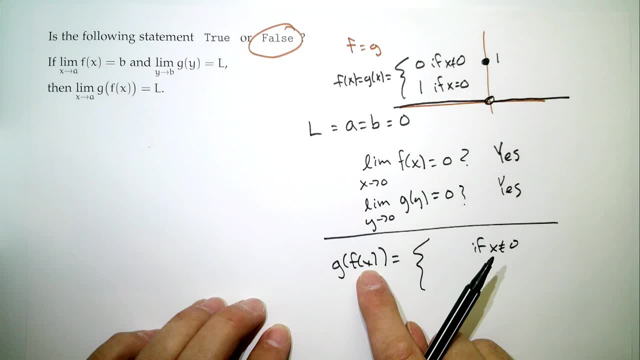 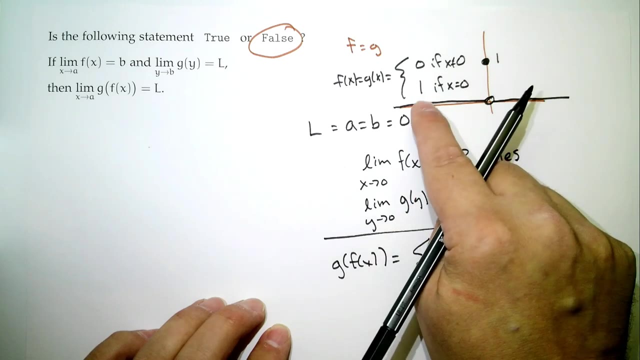 what is the f of 0 going to be? It's going to be 0. And then, with g of 0, it will be 1.. So it's 1. if x equals x is not 0.. If x equals 0,, f of 0 is 1, then g of. 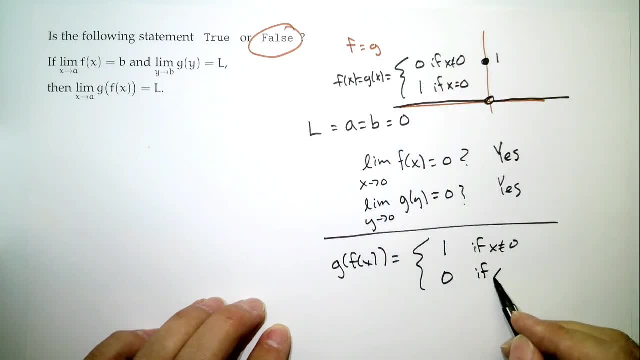 1 is 0.. So it's 0 if x is 0.. So if you sketch that function, it has a very different shape. It looks 0 here and then it's a flat line up here. So the question is: what's the limit? 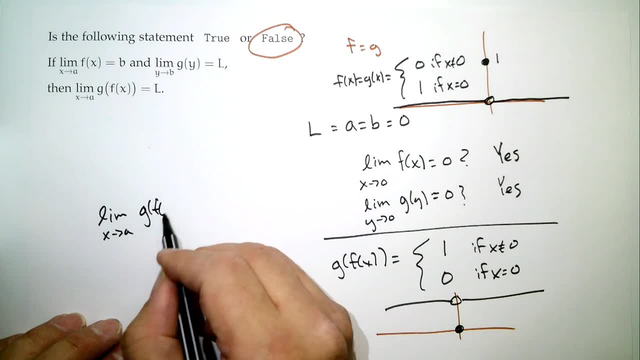 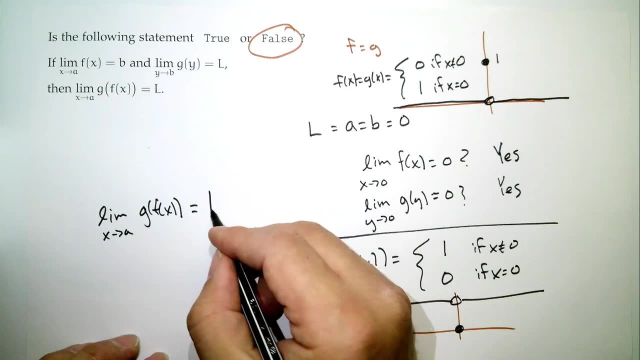 as x approaches a of g, of f of x. Well, what value am I approaching? 1. Notice, that is not l. Okay, now, at this time, you're probably thinking. you know, this is the kind of reason why mathematicians don't get invited to parties. But you're right, because we like to think. 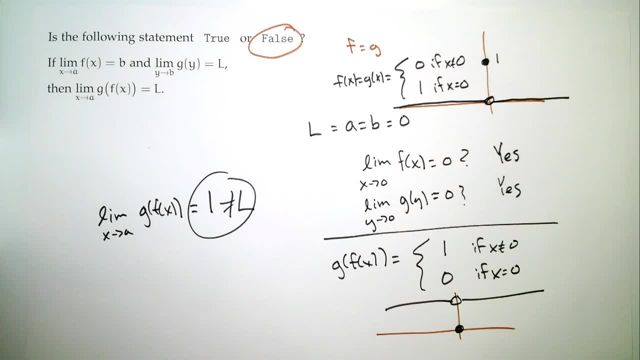 about things and we have to be very cautious. Now, where did our sort of our intuition fail us? And the problem is that we were dealing with a particular phenomenon, which we're going to talk about today, But here's where our intuition fails. You see, what we're talking about is, when we talk about limits, we always 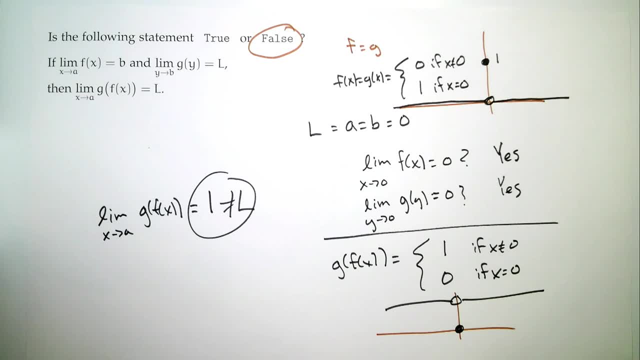 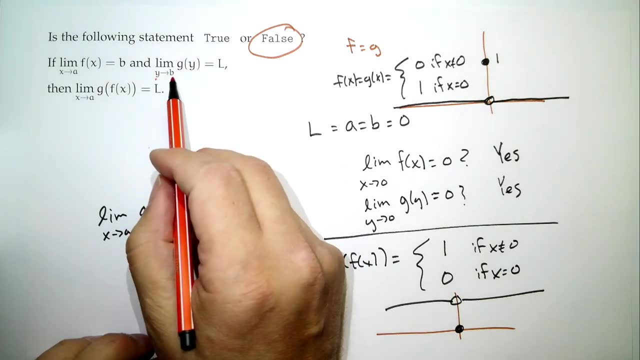 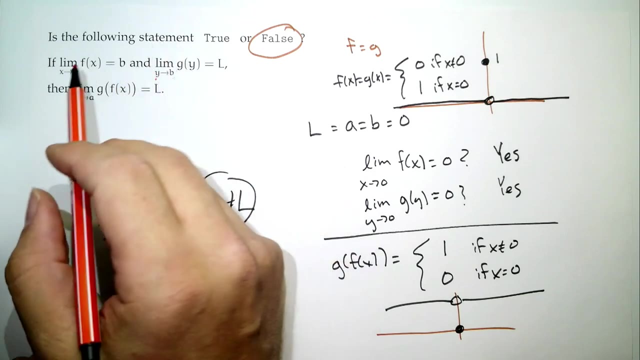 say, well, what's happening nearby? And we ignore what happens at the point itself. And so here what I'm saying: as y gets close to b, well, it can't be the value of b, It has to be near b. But what was happening when we looked? 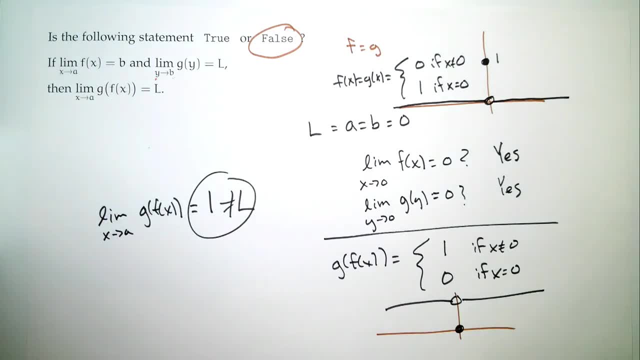 at this output. the output was exactly equal to what b was, so that we were putting into something. our f of x was plugging in something which was not allowed. So that was the issue. Now, the good news is, this is a very subtle thing. We're not going to make anything this. 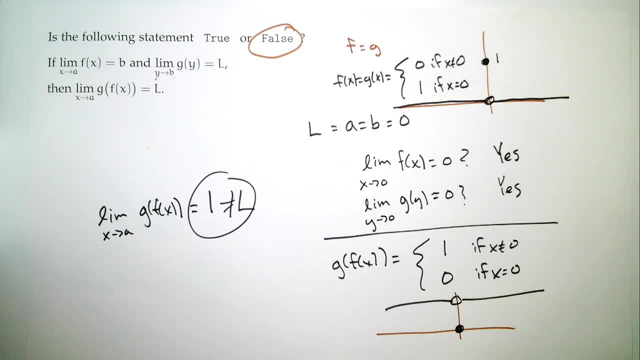 subtle going forward and we're going to fix it. So what's the problem? Well, the problem is you had this issue where you had something weird happen and, in particular, when we say something weird happened, is that sort of what you want to be true didn't match with what happened. So, in other words, your 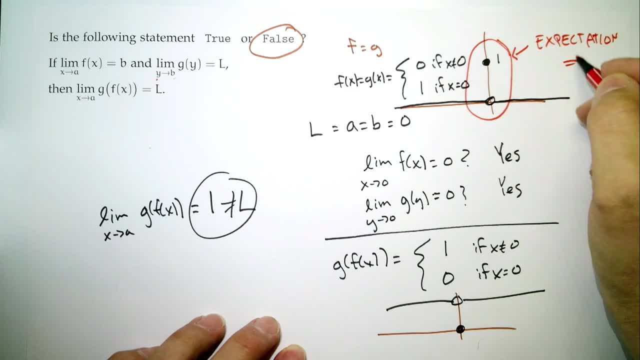 expectation did not meet reality. I'm sure there's some correlation to dating apps these days, where expectation is not the same as reality. 54. to say: look, let's try to avoid that. And here's the beautiful thing, If you can get. 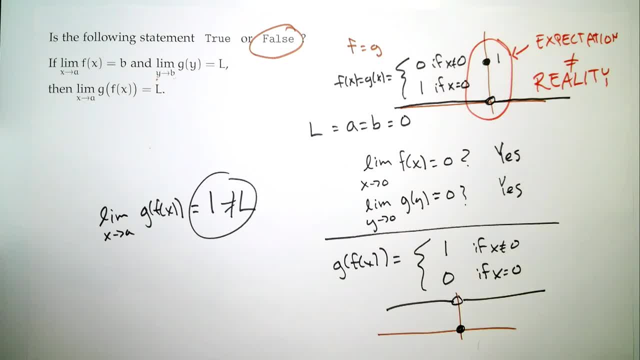 to the types of functions where expectation and reality line up, then this statement is completely true And that's why most of your instructors, your graduate students you talk to, that's why they think the statement is true, because they always will implicitly say: oh, 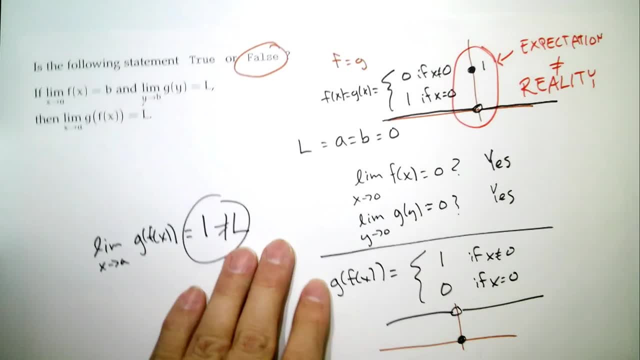 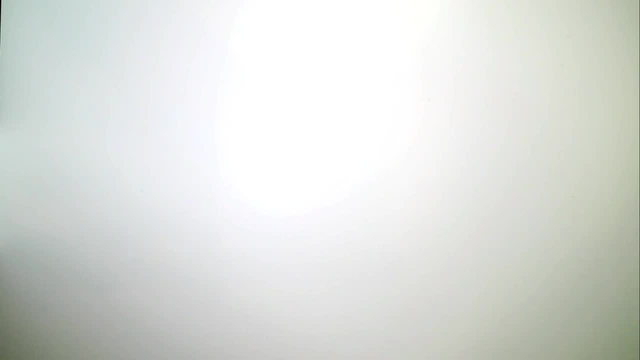 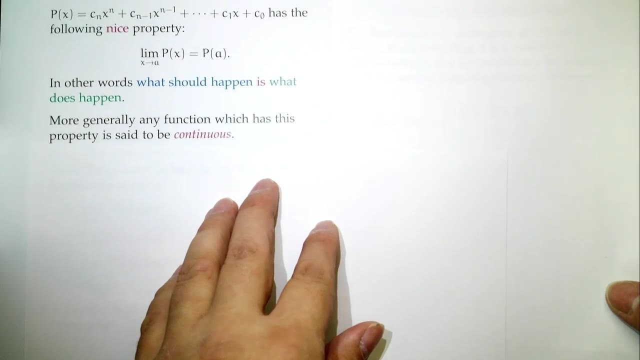 it's a nice function. So that's our topic for today. What do we mean when we're talking about this word nice function? So let's start with the nicest functions that we know, and that is polynomials. So polynomials have this lovely property in that. 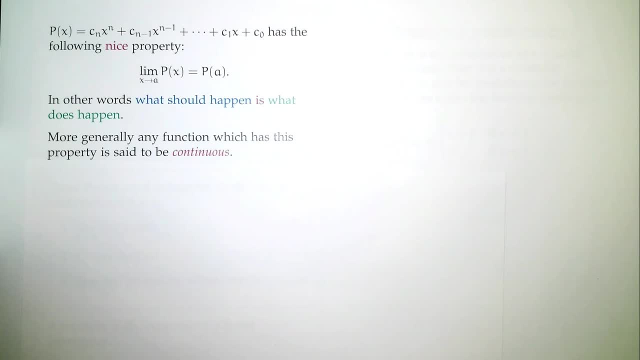 we showed that if I have any polynomial, and that means powers of x combined together in a nice way, that if I want to understand the limit of that polynomial all I have to do is to plug it in. So here in polynomials we have the case. 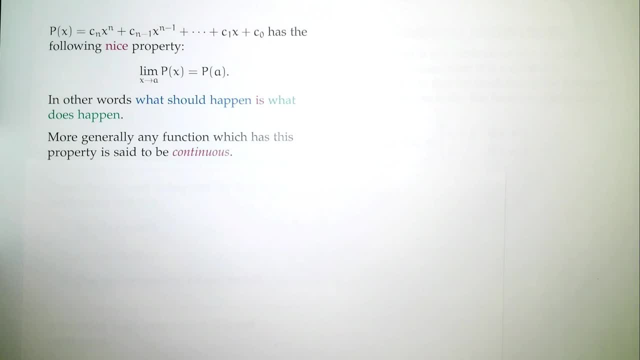 we have the case of what should happen is exactly what does happen. So when we have that, that's a really nice function, and we give a name for this type of function. These are called continuous functions, And these are the types of functions that we're going to encounter. 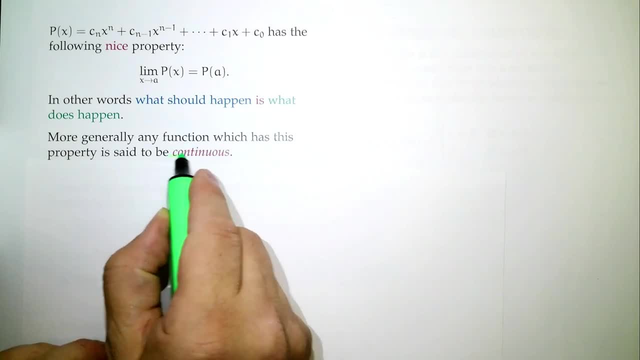 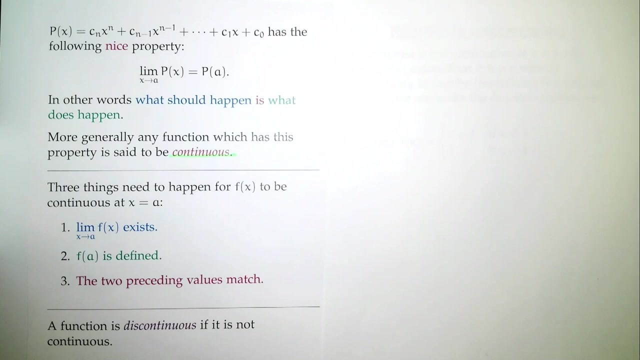 when we're doing our math mags. And it's good, because most of the functions you encounter out in the wild will be continuous functions. So what needs to be true? Well, if I have a continuous function, there has to be three things that hold. 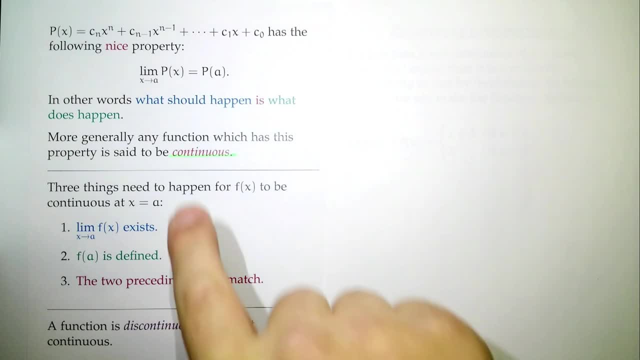 Because what needs to be the case? Well, first off, I have to talk about the limit. If the limit doesn't exist, I can't talk about continuity, So the limit has to exist. The second thing is that the function has to be defined, because I 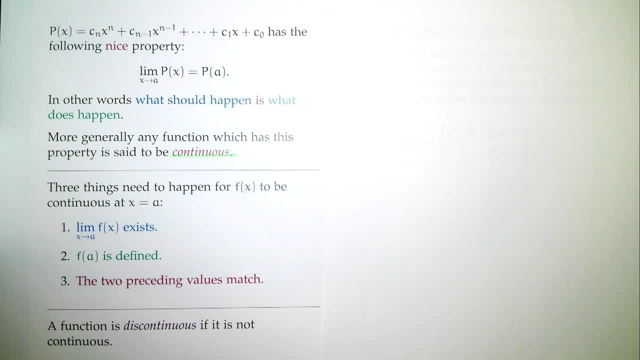 need to be able to plug into the function. And the last thing is that those two values, the limit and the actual value of the function, have to agree. So again, the limit has to exist, the function has to be defined and those answers have to match. So that's what it means for a function. 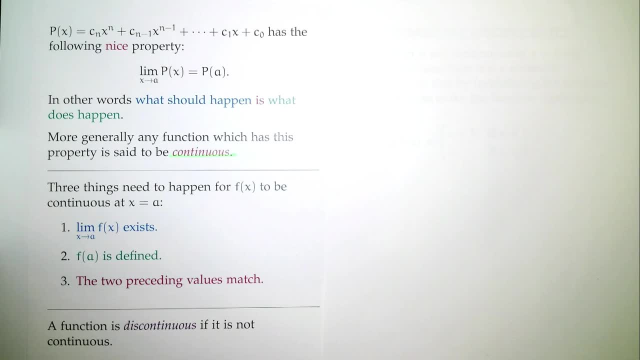 to be continuous, And if a function is not continuous at any particular value, we say it's discontinuous at that location. Alright, Well, what kind of continuity problems can we have? It turns out there are several different things that can happen. 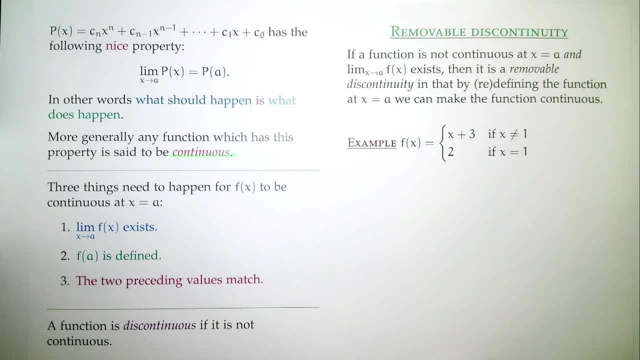 We're going to talk about a few of them and we're going to give them names. So the fact that we have different names means there's different types of phenomena. There's two in particular that we need to sort of deal with. So the first type of discontinuity is what's called the removable. 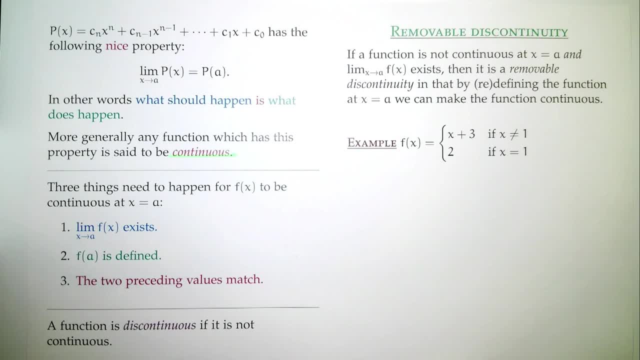 discontinuity. Now what is that? Well, the function is not continuous at x equals a, but the limit exists. So see if the limit exists. if you think about these three criteria here, the limit existing is sort of the hardest one to do, because limits are pretty tough. 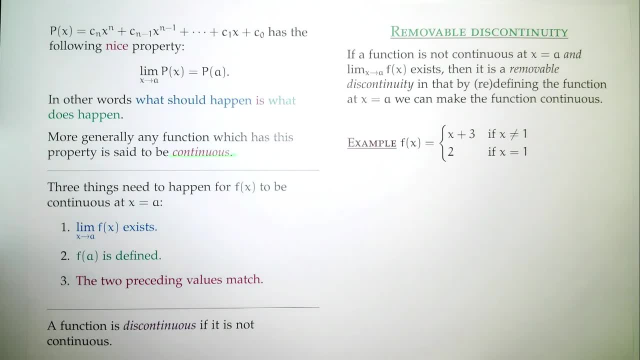 But if the limit exists, we can say: look, we can patch it up and make it work. And we do it by saying: okay, what do we need to define the function to be in order to make it continuous? So here's an example. I have this function f of x. 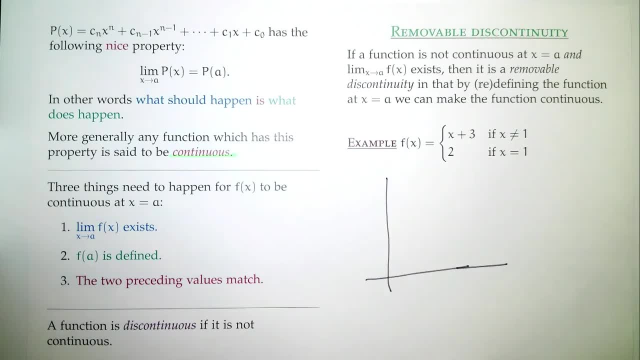 which is x plus 3, if x does not equal 1, and it's equal to 2 if x does equal 1.. This is a pretty simple function, because x plus 3, that's a line, And it's a line we can mark it. the intercept is at: 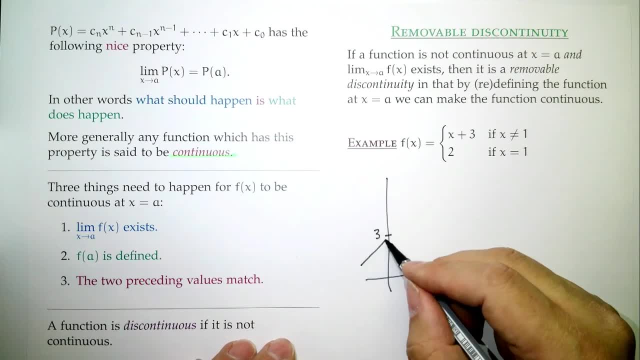 3, the y-intercept slope of 1.. And the only catch is that's if I'm not 1.. So at 1, there's something different. So I'm going to put a little circle here indicating that that's not what happens. 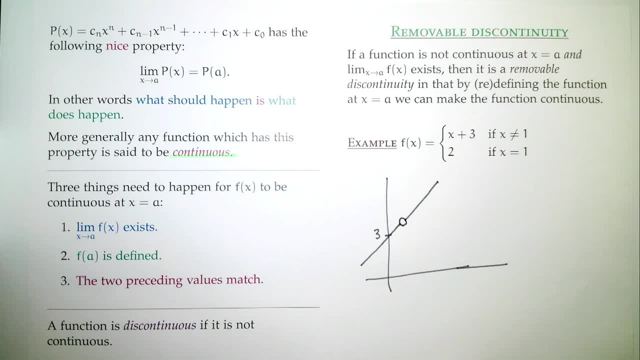 at 1.. At 1, what happens is we get a value called 2., Which is down here. So this is a discontinuous function. Now I claim it's discontinuous. We should check what is the limit as x approaches 1. 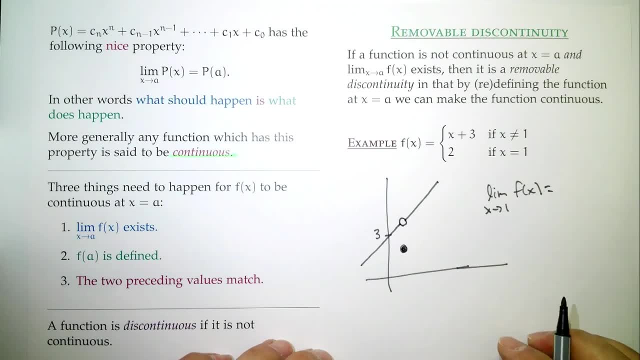 of f of x, It's 4.. Because if x approaches 1,, what we can do is we can say that I can replace f of x now by this expression x plus 3.. Because as I approach 1, I'm not 1, so I can use that rule And then that's. 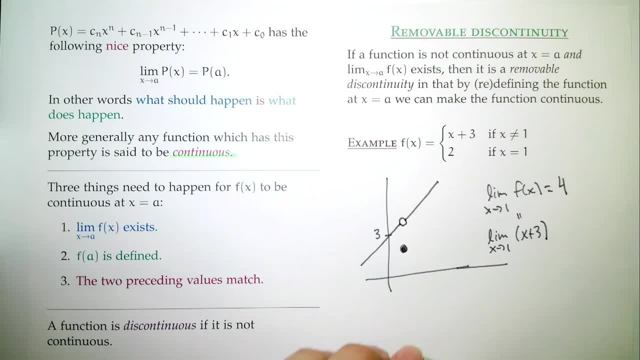 a polynomial, that we can take that limit. But of course this 4,, it turns out, does not equal 2.. That's one of those cool facts you learned back a few years ago. And that's f of 1.. So this is not continuous, but the limit. 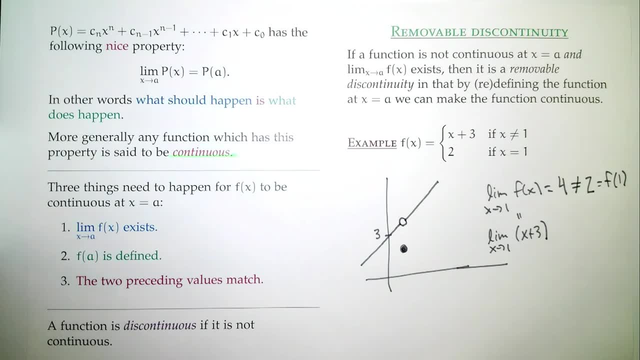 does exist. So how do we fix our function? Well, the easy thing is to say: that is in the wrong place, So we just want to move it and fill in the hole. So we say, alright, well, what should we make it? And the answer is: whatever the limit. 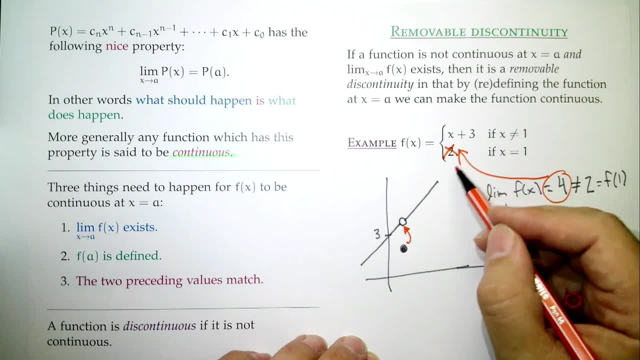 turned out to be. that's what goes here, So we replace the 2 by 4, and now our function is continuous. Of course, you might say: well, there's a much easier thing, Just call it x plus 3 everywhere. 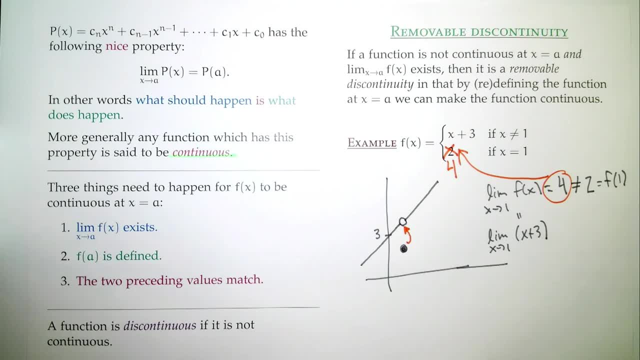 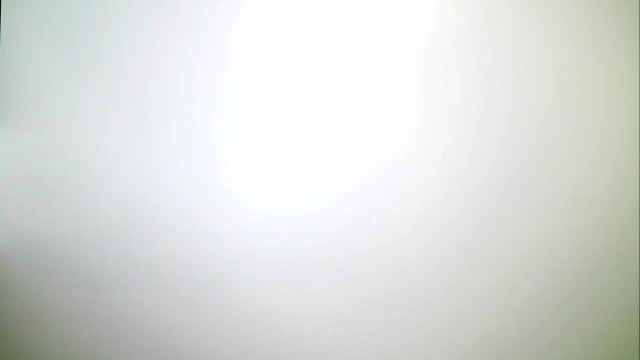 And that's true, because this is a simple example, But we might have something more interesting, So let's do a different example. that's more fun, Alright, So here we go. How should the value a be chosen so that the following function is continuous at t equals 0?? 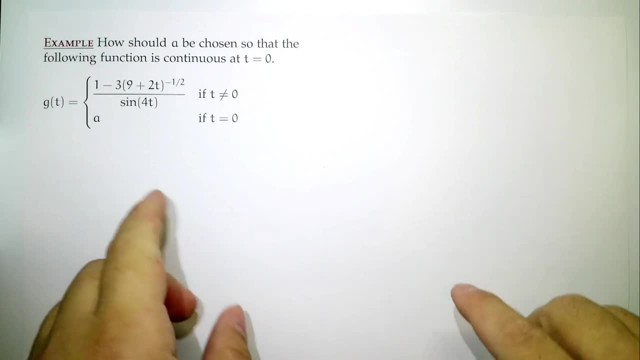 So we have this function g of t. It's again a piecewise function. Now we don't know what it is at 0 yet, so it's some number a. We've got to figure out what a is, And then there's this sort of 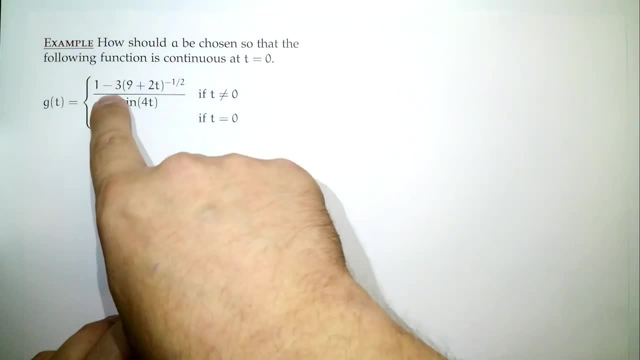 weird looking other expression: 1 minus 3 times 9 plus 2t to the power of 3. It's a negative 1 half over sine of 4t. Huh, Hmm, Well, that does not look fun. But. 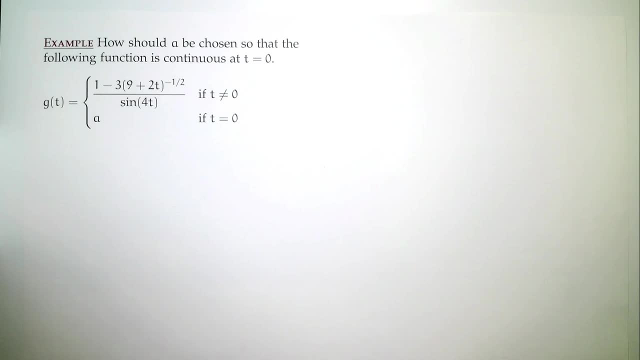 we're going to do it anyways. Alright, Because we've got to know Inquiring minds. Now, one thing that's tempting to do is just plug in 0. And if you plug in 0, well, you'll get sine of 0 downstairs, and that's always a dangerous 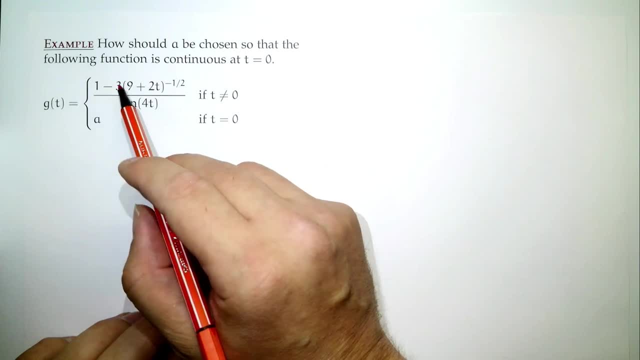 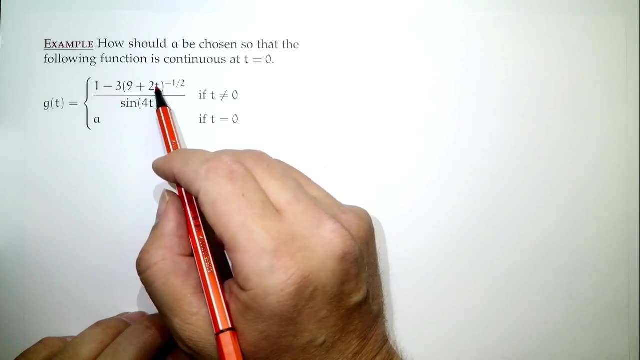 thing Upstairs, you're going to get 1 minus 3.. Then you're going to get 9 to the negative a half. Now the negative really means like 1 over, So it's like 1 over square root of 9.. 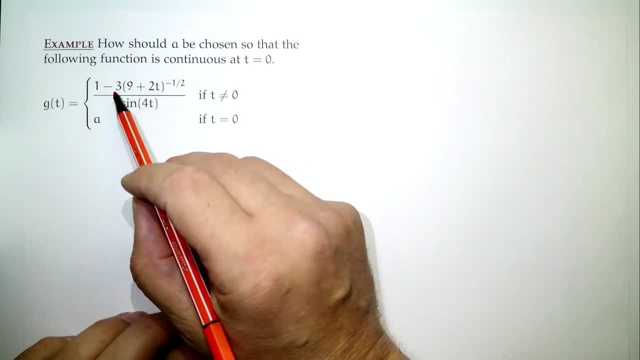 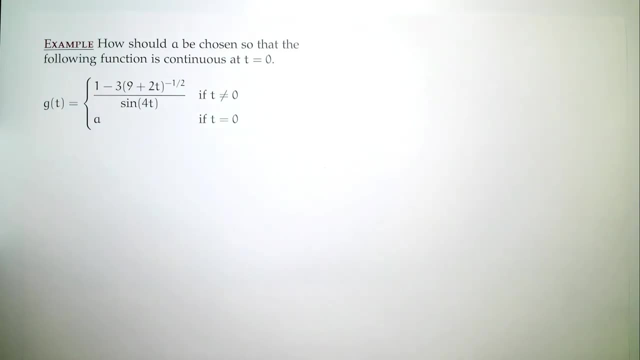 Which means this part, there is a third, 3 times a third is 1.. And so we're getting 0 over 0.. And if you see 0 over 0, what do you know to do? More work, More work, Alright. So. 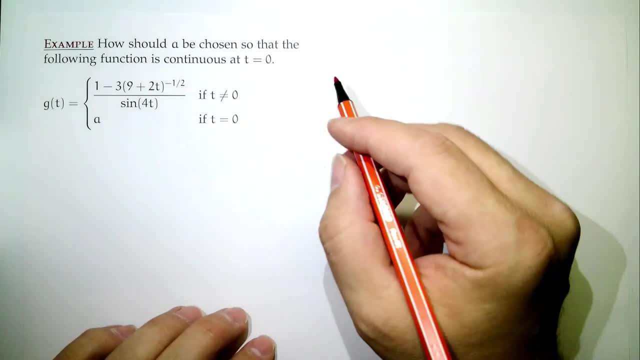 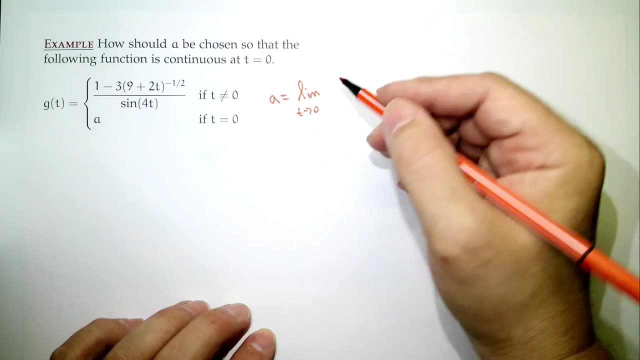 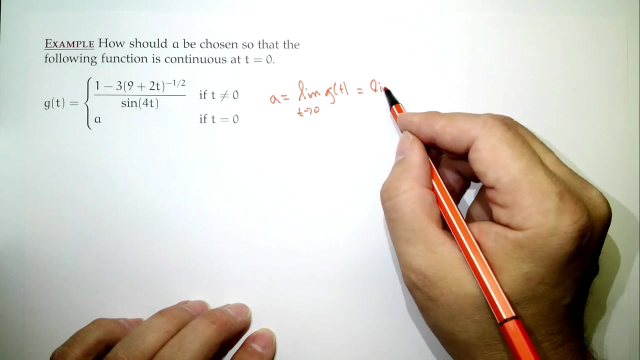 here we go To figure it out. what should a be? Well, the answer is: a should be, whatever the limit is, as t goes to 0 of our expression g of t. Well, of course, what does that mean? So we say: this is limit as t goes to 0.. I can. 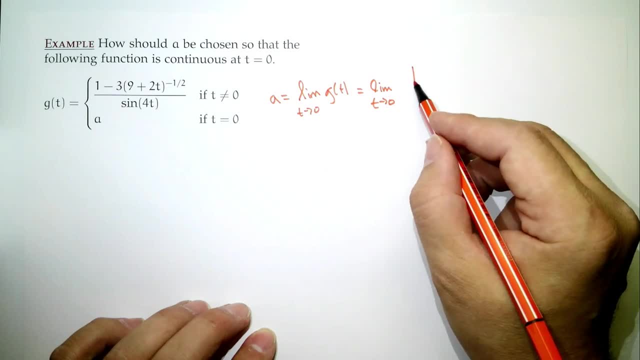 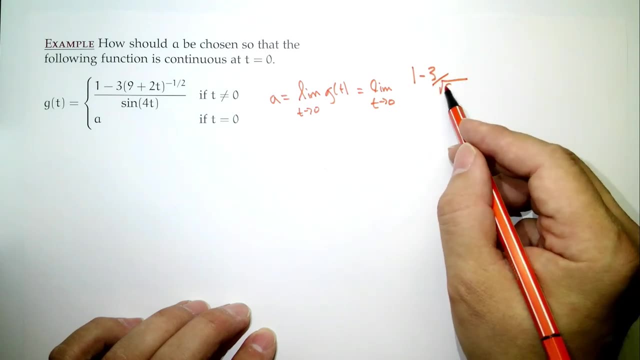 plug in this expression here And we're going to clean it up. Instead of writing it as 9 plus 2t to the minus 1 half, we'll write as a square root of 9 plus 2t downstairs. So 1 minus 3 over square root of 9 plus. 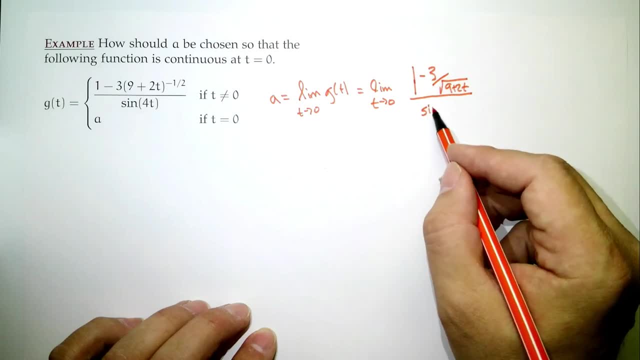 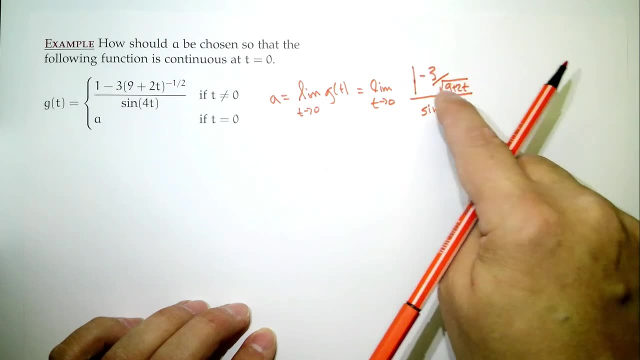 2t, Alright, And then we have sine of 4t And I don't like sort of a fraction within a fraction, So I'm going to replace this one, This one in front. we can write that as square root of 9 plus. 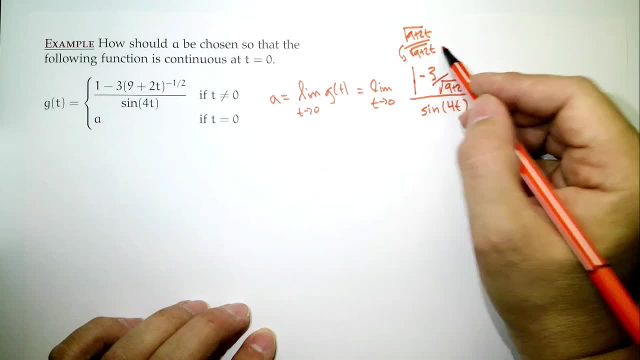 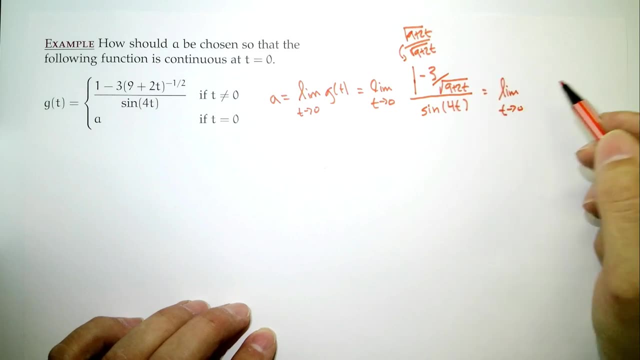 2t over square root of 9 plus 2t. So we're getting a common denominator. So if we do that and we move that square root of 9 plus 2t downstairs, then we have that this expression is the square root of 9 plus 2t. 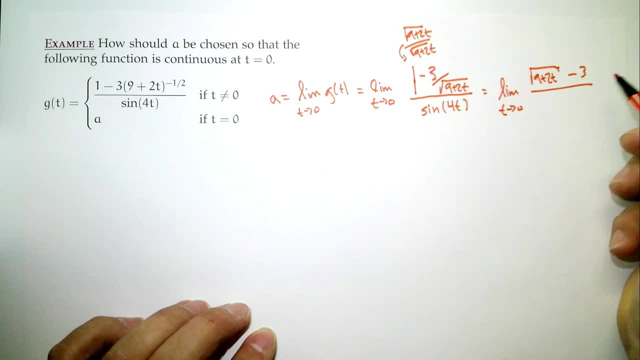 minus 3 over well sine of 4t and the square root of 9 plus 2t. Alright, So that's just a little bit of gentle massage. Now we still have the same issue. We still have 0. 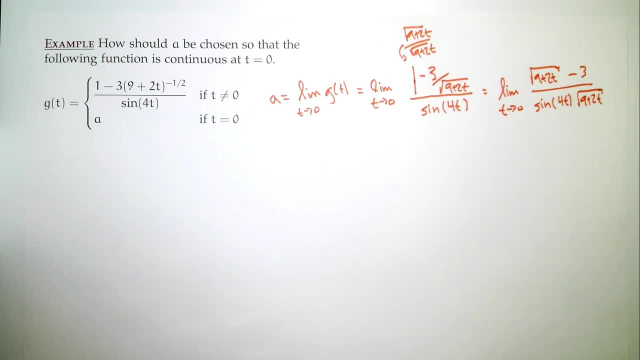 over 0.. We haven't really cancelled anything. We've found a way to say: aha, this 0 over 0 we can handle in a nice way. The fact that we see a sine function makes us say it'd be really cool. 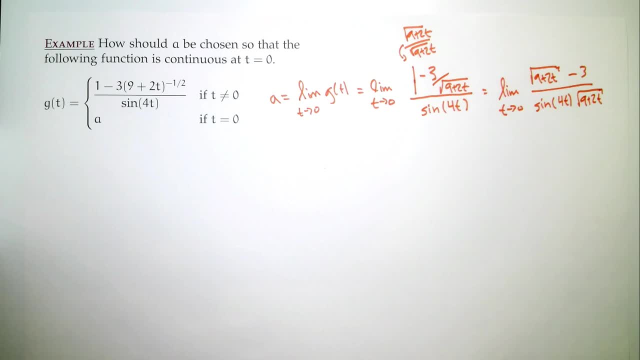 if I get like a t or a 4t somewhere in there, Because I know that sine of blah over blah is 1. Well, hmm, don't have that yet, But well, we're still early in the problem. So 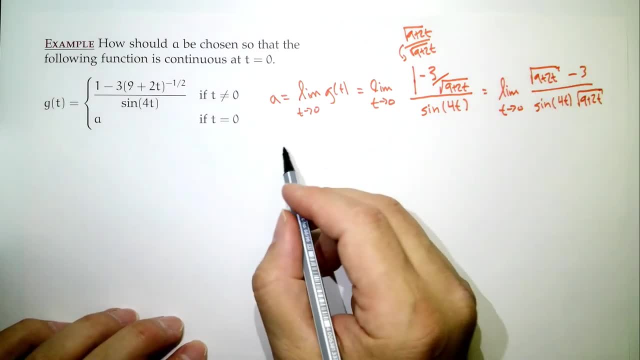 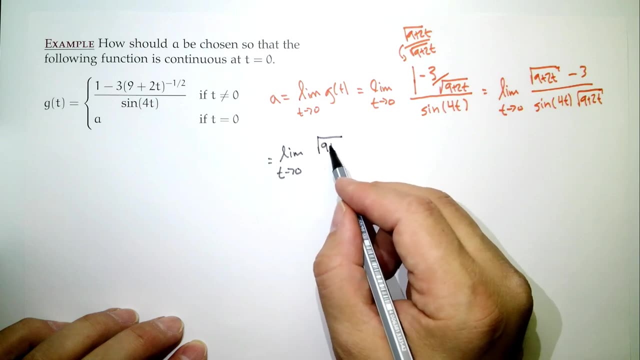 the next thing is to say: we have a square root. So what do you do? if you see a square root, Conjugate- Yeah, conjugates are really useful for getting rid of squares. So we have our expression and when we say conjugate, we're going to multiply. 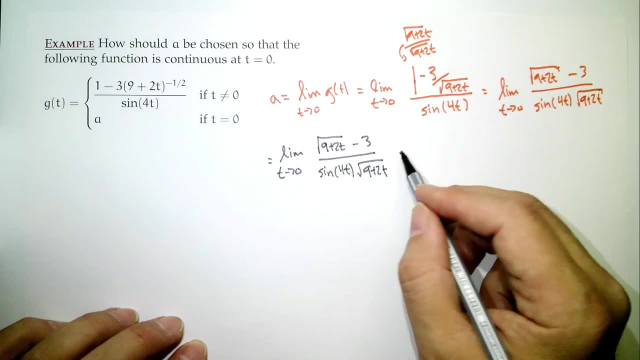 both the top and the bottom. So if we think of this as a minus b, we're going to have a plus b, a plus b, Alright. And now upstairs. well, when we multiply that, we're going to get a squared minus. 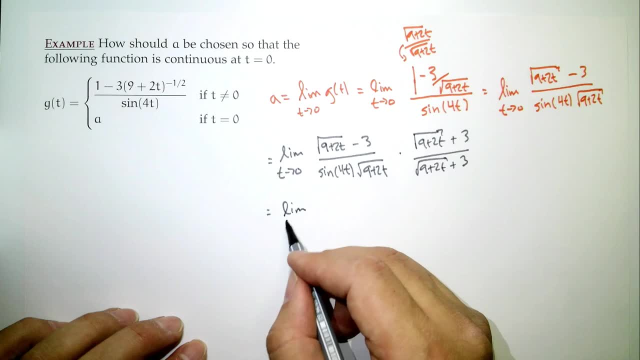 b squared, So that becomes the limit as t goes to 0. We're going to get 9 plus 2t, That's a t Minus 9.. And downstairs, don't multiply it out On the part that the conjugate's. 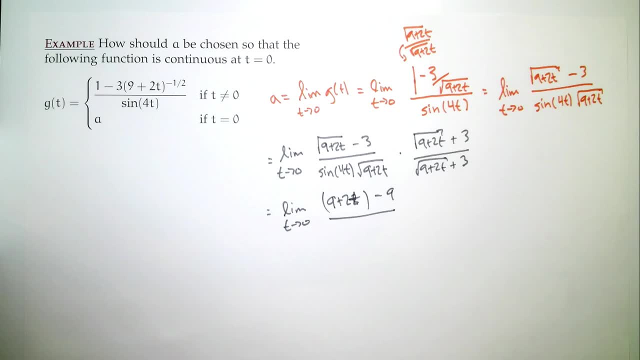 being useful for: yes, multiply it out. On the part that it's not useful for, don't, Don't multiply it out. Leave it as it is Okay. Sine of 4t, The square root of 9 plus 2t. 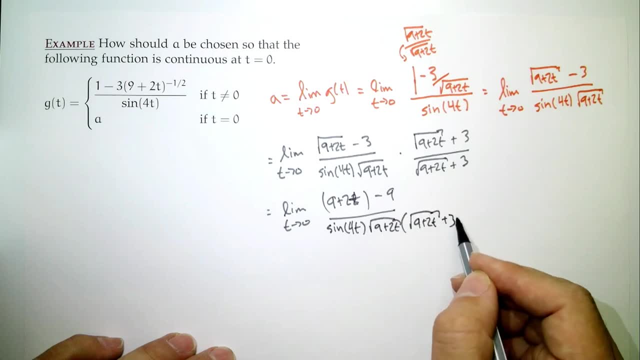 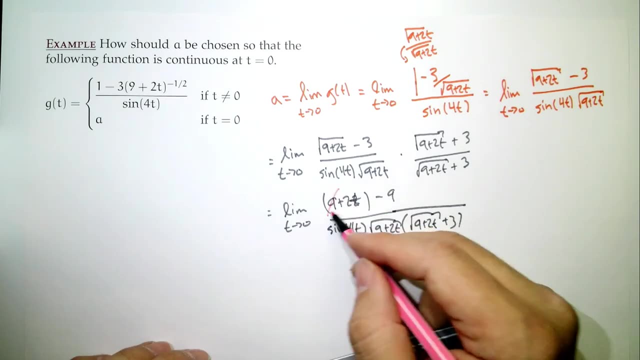 And that square root of 9 plus 2t plus 3.. Great, Now from here we're like: hey, good news, The 9's cancel out. So we're making some progress And we also have some other progress. 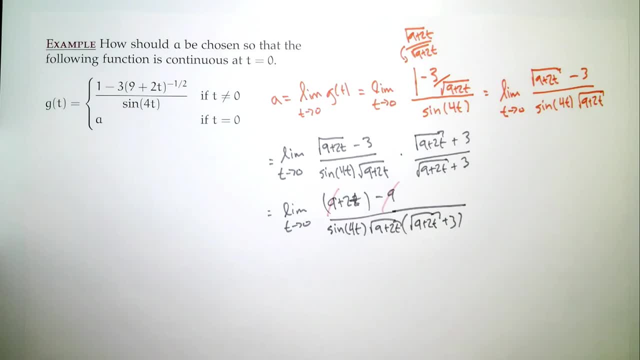 So we have a nice fact here. Let's recall the limit as law goes to technical math term: blah, But sine of blah over blah. Do you remember what that is? Yeah, Okay, You've mastered it. What if we did the following? It's still. 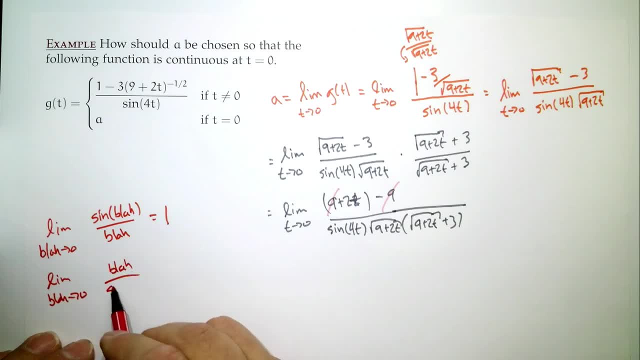 blah. but we did blah over sine of blah. It's still 1.. Yeah, Because if you take, you just flip the limit as well. So I say, hey, you know, I've got like sine of 4t. What would be great. 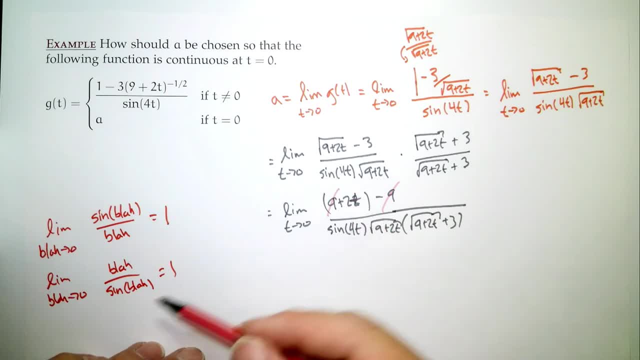 to be upstairs 4t, Because that would get us right into that nice sweet spot. We're close. We've got 2t Because the 9's are gone. How can I make it 4t? Well, the 2t we already have. 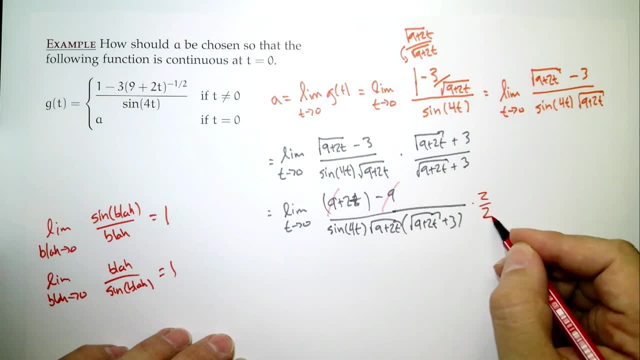 So we just need the 2.. So we're going to multiply by 2 over 2.. So this is the limit, as t goes to 0 of 4t over sine of 4t, And then everything else. 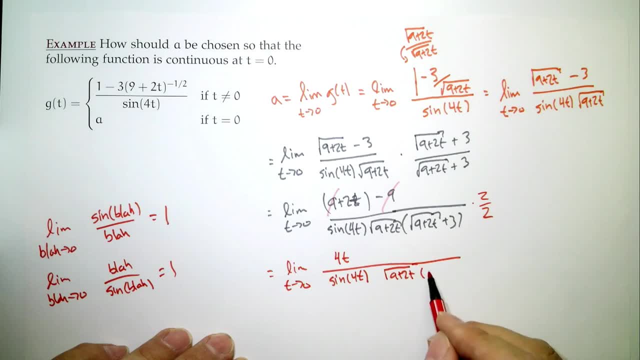 Square root of 9 plus 2t, Square root of 9 plus 2t plus 3.. And there's a single 2 coming from right there. So at this point, what we like to do is we like to sort of group And we 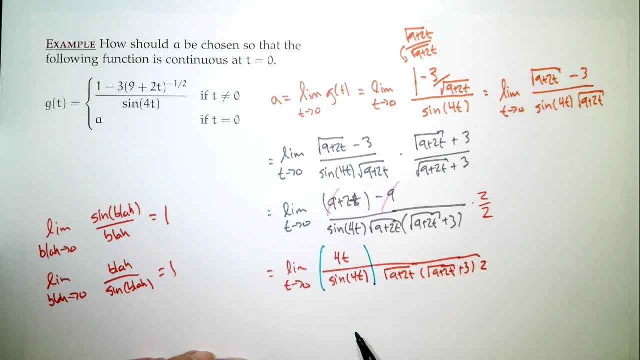 say that 4t over sine of 4t, it's a blah, something sine of blah. The inside of the sine matches the other part. What does this single part go to? It goes to 1. And sort of the philosophy here is to say: 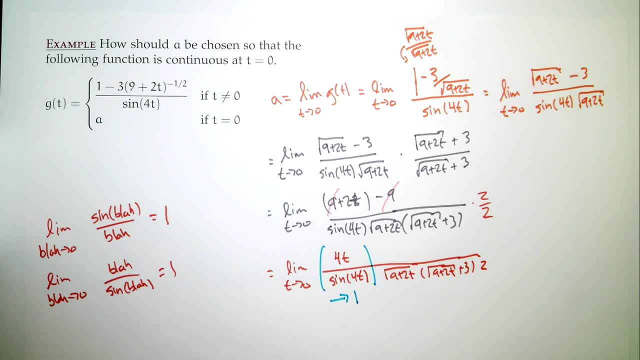 if you can break it up into parts and you know the limit of each part, then you're fine. So what we did, was we manipulated to the point where we said, hey, that 0 over 0, I can put in as being something over the sine of. 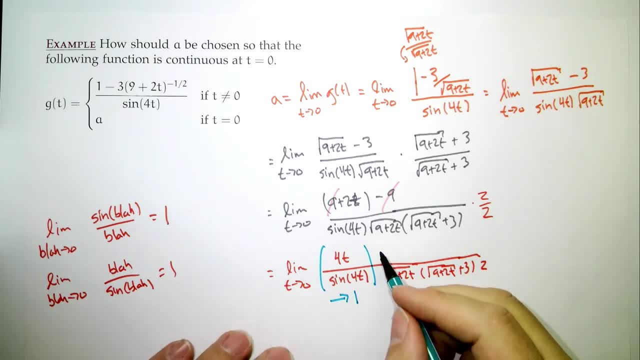 something And that part I can manage And therefore I have everything else. Now the hope is: this goes to something. Well, the top is 1.. Then you go, let's work through the terms: Square root of 9?. 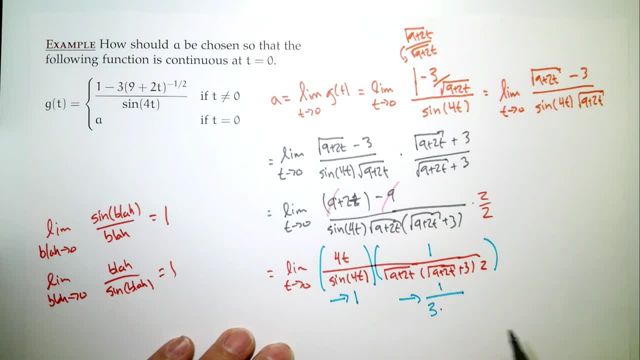 3. Square root of 9 plus 3? 6. And 2? 2., Giving 1 over 36.. So the answer is that A should be 1 over 36. And if that's what you pick, then 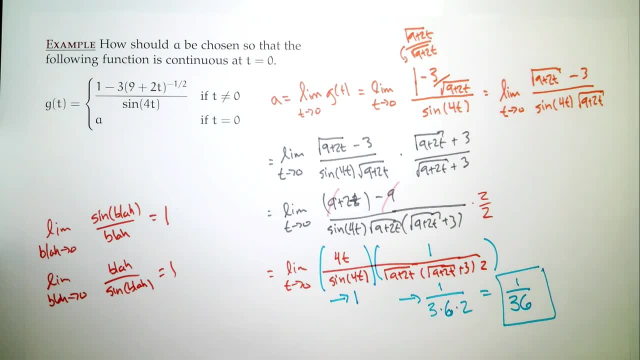 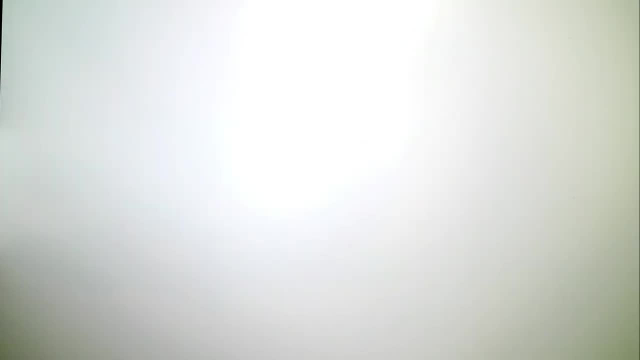 your function will be continuous. Okay, so that's an example, That's if we have our limit existing. Now there's another type of discontinuity, which is the following: It's called the jump discontinuity And it says: suppose 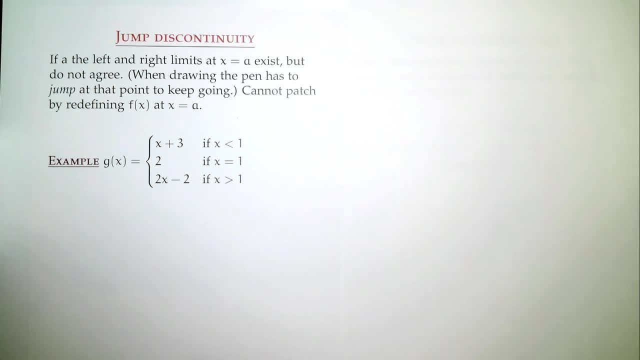 Oh, there's a typo here. I should have fixed that. Ignore that A. So if the left and right limits at x equals A exist but aren't the same, then it's called the jump discontinuity. And where does the name come? 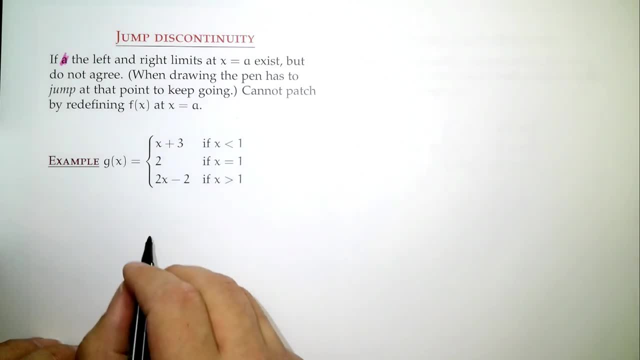 from: Well, if you sketch it really quick. so let's do an example. I claim this as a jump discontinuity. So I have x plus 3 if x is less than 1.. So that looks something like that. 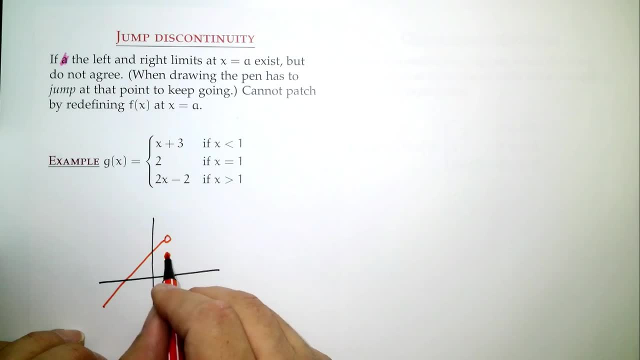 I'm at 2 if x equals 1, which I'll say roughly there, And I'm 2x minus 2 if x is greater than 1.. And that looks something like that. So this is what 3 of x looks like, if you were to sketch it. 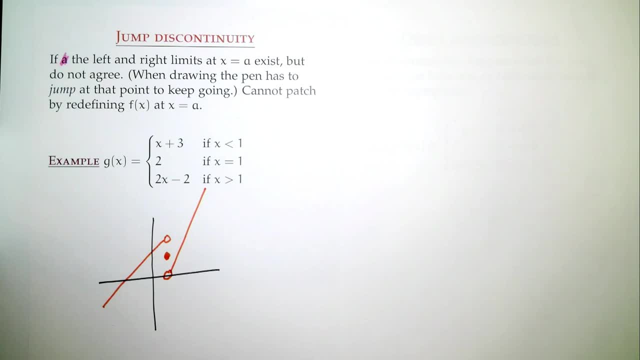 Now, what's happening here? Well, when we come in from the right- on a side note- this is 4.. When we come in from above, from the right side, we're approaching 0.. When we come in from below, from the left side, 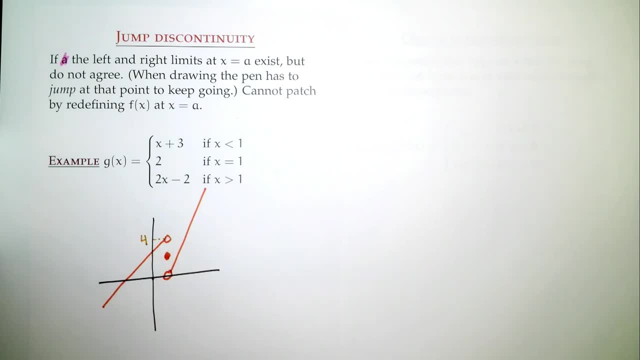 we're approaching 4.. And 0 and 4 don't match. We can see the picture. So the jump is: suppose you were trying to draw this with a pen or a pencil As you're drawing, and then you get to this point 1,. 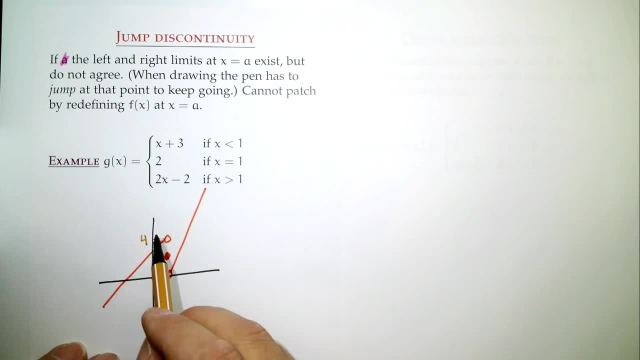 you have to jump up, lift the pen or pencil and then start drawing again. Now here's the issue: Removable discontinuities you can patch, because it's just like you've got to fill in the hole. Jump discontinuities you cannot. 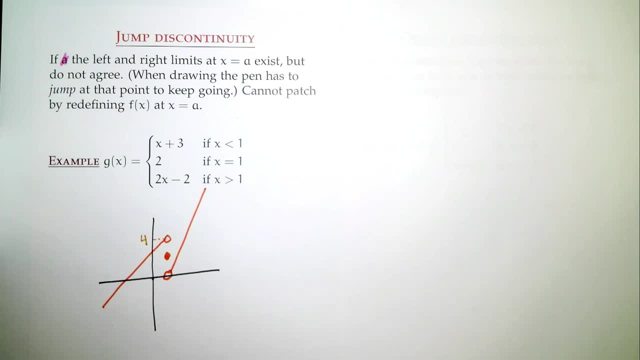 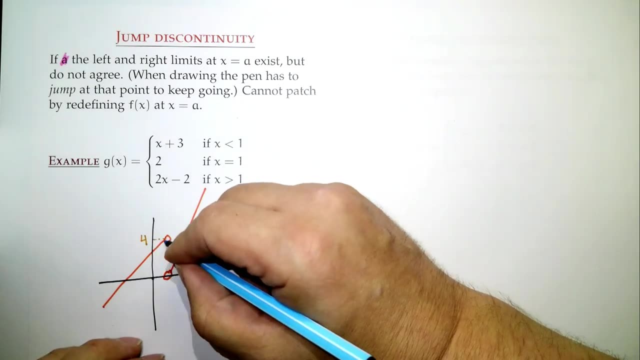 patch them up. There's no way. There's not a huge patch. You can't say: aha, I know, Here's an idea that Steve hasn't thought of. I'll just make like a really large patch. No, no, no. 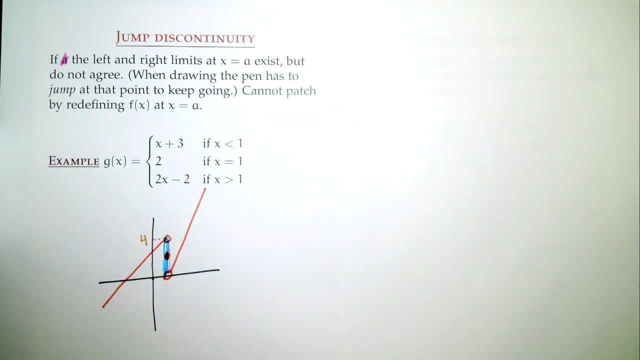 You can't do that. So a jump discontinuity is something which you cannot make continuous by redefining. So that's what a jump discontinuity is. There are other discontinuities and essentially the other discontinuities fall into the category of. 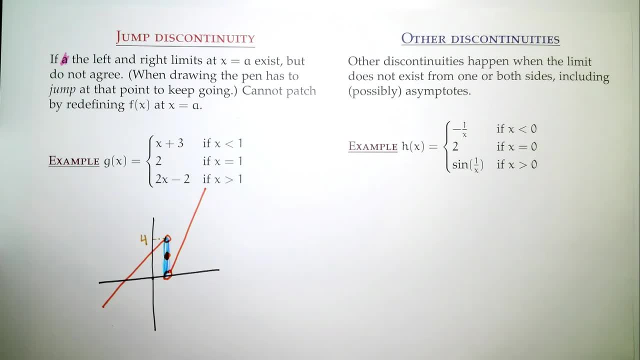 the limit has a problem, And there's lots of ways for limits to have problems. One thing is that it might blow up. Another thing is it might have some infinitely many functions, and so forth and so on. So an example of this: if you 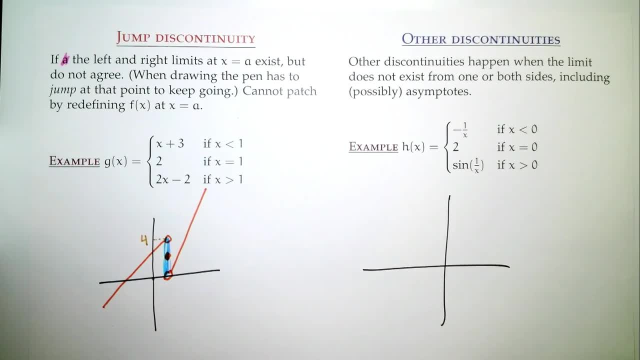 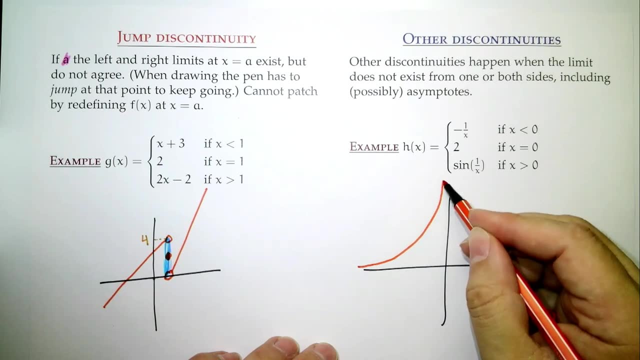 were to look at this function. here's this h of x. When x is less than 0, it looks like negative 1 over x, which means that as you get close to 0, it's blowing up, So it's going towards infinity. 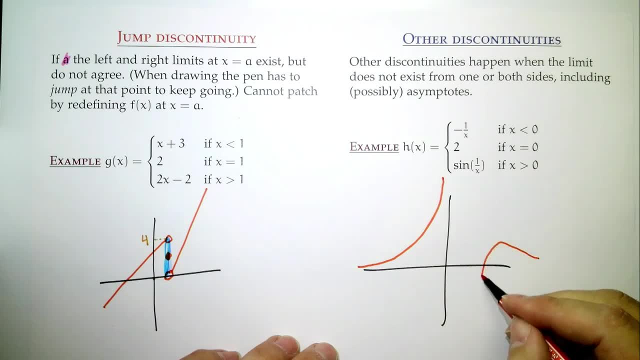 From the right it looks like sine of 1 over x, which is a very fun example, just because it has that ability to oscillate and we can actually understand it. and then, of course, at 0,. well, for some reason it's been. 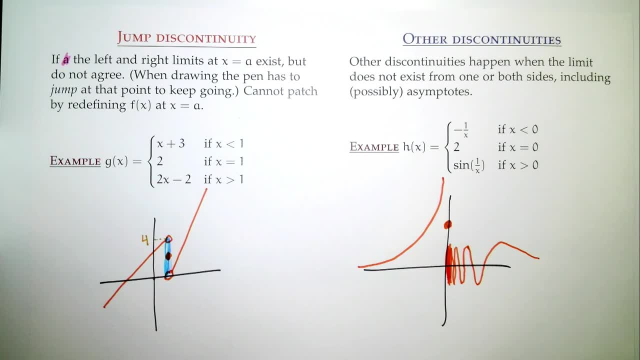 defined to be 2.. But you can see that this has- it's a limit, with some very serious problems. The limit doesn't exist. Now you might say, well, couldn't we say that the limit from the left is infinity? 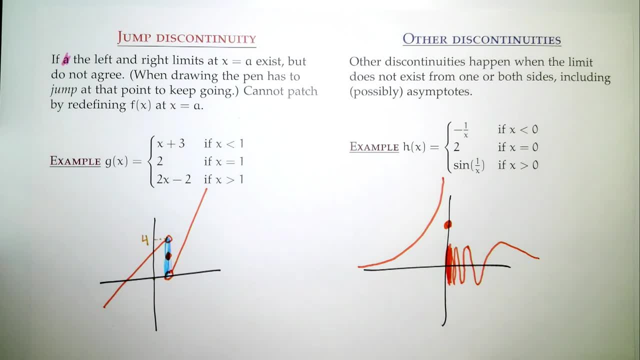 And that's a great discussion which we're going to have very soon, but not today. So there's our two big types of discontinuities to be aware of. You've got your removable, you've got your jump, then everything else is sort of like: 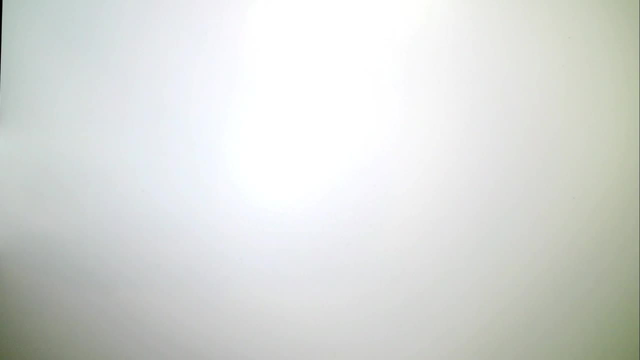 well, there's problems with the limits. So we say that a function is continuous if the function is continuous at every point. So one of the things we might want to do is say, well, let's make it a continuous function. So here's a. 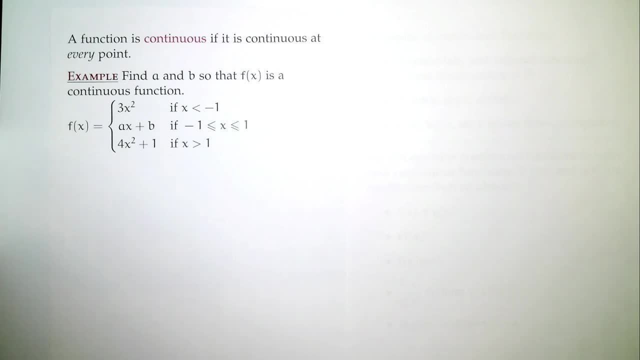 nice example. Find the values a and b so that the function f of x is a continuous function. So we want this to be continuous. So our function has three parts. If I'm below negative one, I look like three x squared. If I'm between negative. 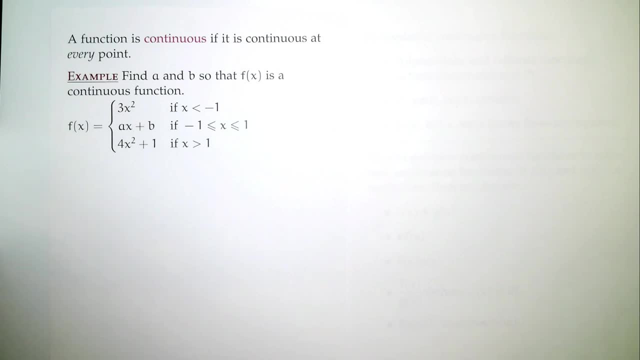 one and one. I look like ax plus b, where a and b are to be determined, And if I'm above one, I look like four x squared plus one. Now, we can sketch parts of this pretty easily. We can certainly sketch. 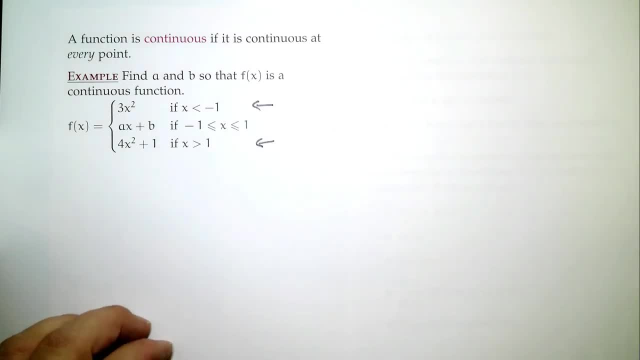 the below negative one and the above one, because they have nothing to do with a and b. So if we were to sketch them, we say, all right, well, what do they look like? Well, three x squared. that's a parabola that opens up. 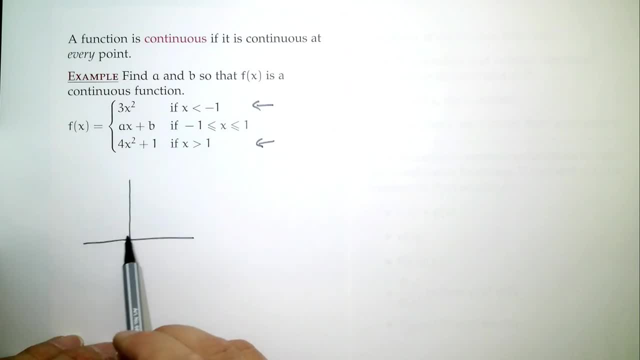 stretched up a little bit. I don't need the whole parabola, though. I just need the part that starts below negative one. So if here's negative one and let's see negative one, I would have been three, So I come up here. 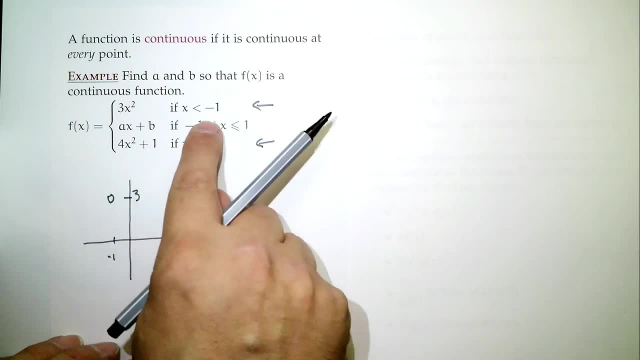 to three and I put a circle because I'm not including negative one, but then I'm coming up off there. So that's the part of the parabola: three x squared, but only the part below negative one For the other side. 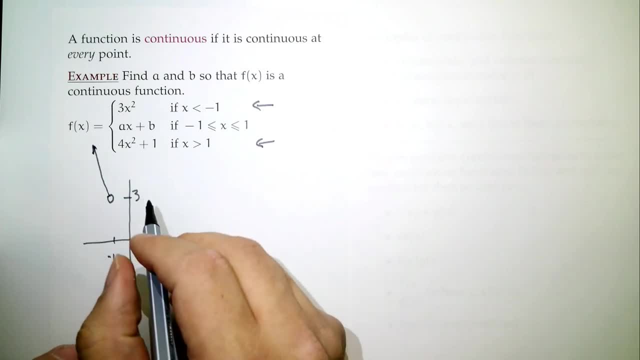 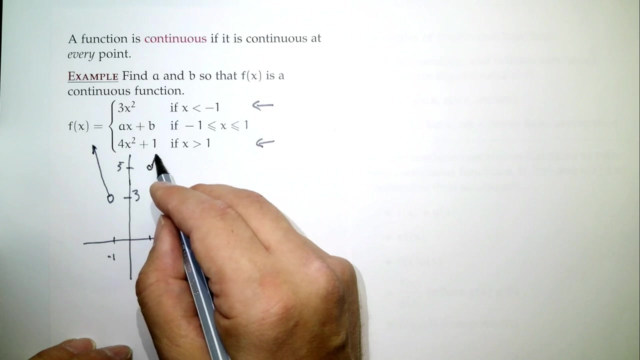 four x squared plus one. what happens? Well, at one I'm going to go up. plug in one. I would get four plus one, which is five, And so that's also going up. Oh, I did not plan well. 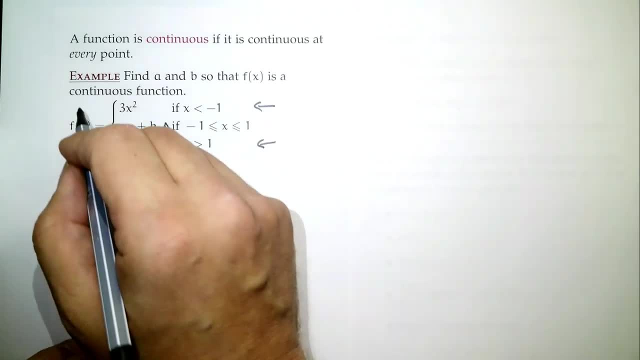 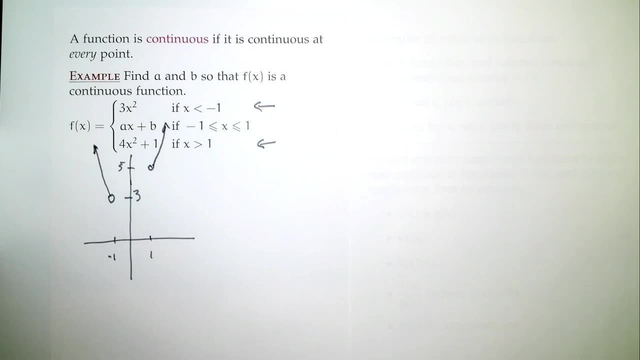 Okay, But again, the four x squared plus one is a parabola, but I only include the part above one. Now I should say you don't actually need to draw the picture to do this problem. I just like to sort of get an intuition of what's going on. 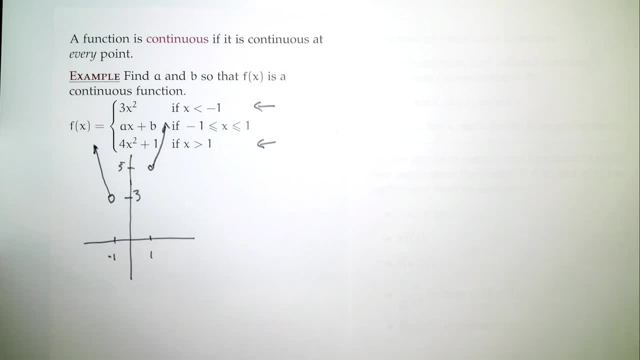 Let's think about the middle. I should pause and say: is three x squared a nice function? Is three x squared continuous? It is continuous. What's special about three x squared? to make it continuous Polynomial? Same reasoning says four x squared. 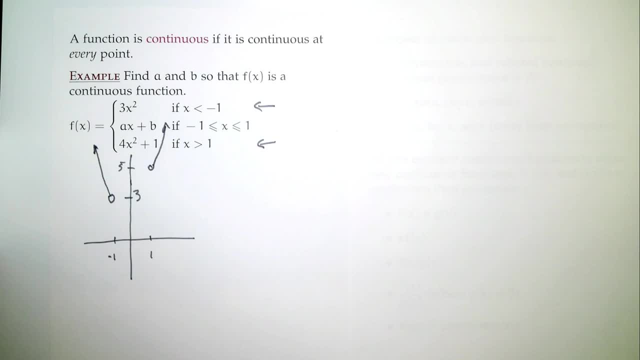 plus one is continuous, So the left part is continuous, the right part is continuous: A x plus b. what does that look like? It's linear or a line? Now are lines continuous? Yeah, So the good news is that each little piece is continuous. 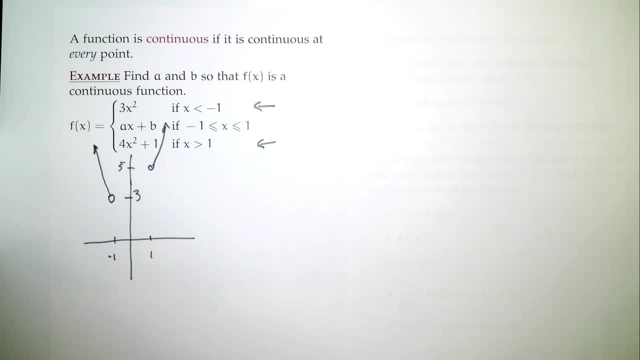 So what do I need to worry about? Well, each piece is continuous. The only thing I have to worry about is where I glue them together. So, in other words, I have to make sure things line up at negative one and at positive one. 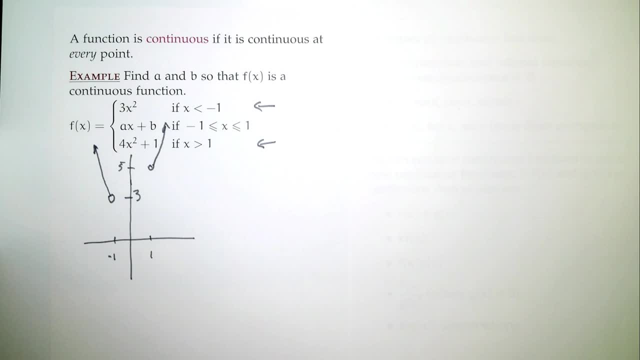 because I'm having two different behaviors from the two different sides. So as long as those behaviors line up, life is good. So how do we figure out what to draw? Well, one thing we can do is we can actually think about in terms of a picture. 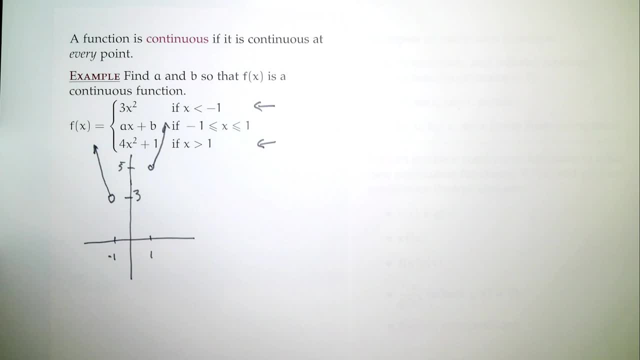 and say: I know I need to put in a line and I need to put in a line that's going to match at these points. So the line has to look like that. It has to be the straight line that connects the point from negative one. three: 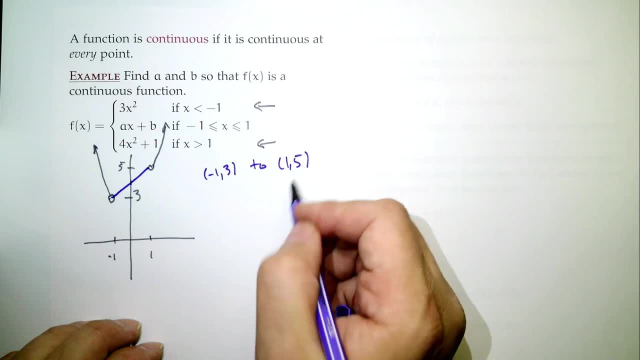 to positive one five. That line segment is the exact line segment that we need. So that's our picture way to see what we need to do Now. once we have that, it's pretty straightforward to figure out what that line is. For instance, what do we see? 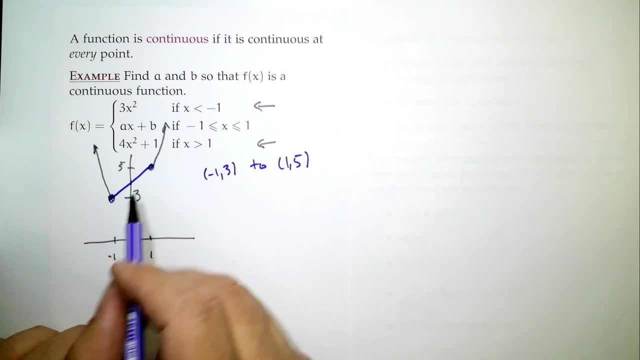 Well, we've gone over to in the x direction, from negative one to positive one. How far have we gone in the y direction? We've also gone two. So what's our slope? Our slope is one, because we went over two. we went up two. 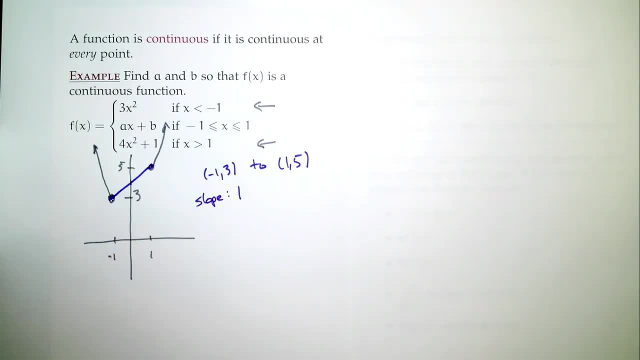 So it's the same change in x, same change in y. Where's the intercept going to be? It will turn out it's halfway in between. because it's nice, because of our symmetry, The intercept is at four, And so our line that we need. 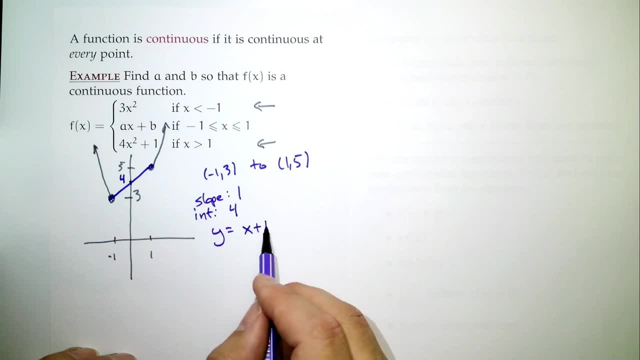 is the line x plus four. So we need to have a equals one and b equals four. Now you might say: could we have done this without a picture? And the answer is yes, absolutely. How do you do it without a picture? 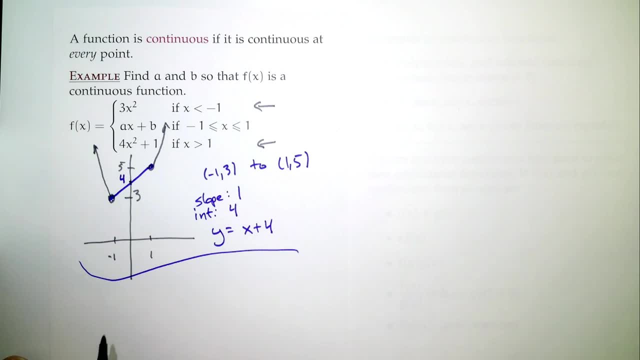 Well, probably give yourself a lot more space. but here you go. We say the only things we need to worry about are negative one and one. So we look at the limits. So limit as x approaches negative one from below of f of x. 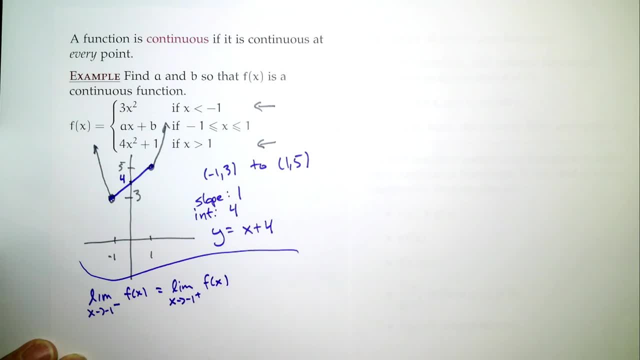 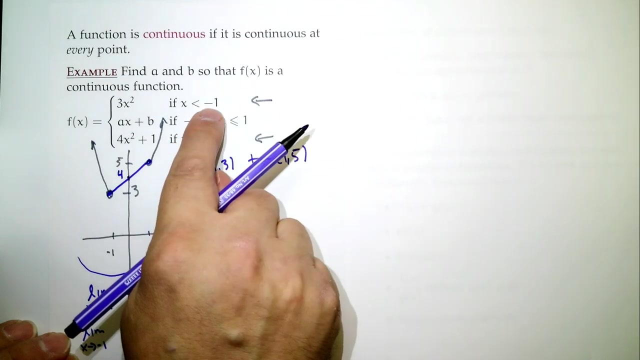 has to be the same as the limit as x approaches negative one from above, so that the two sides agree at where they glue together. If I'm coming to negative one from below, well, I can replace what my function here is, Because if I'm below negative one, 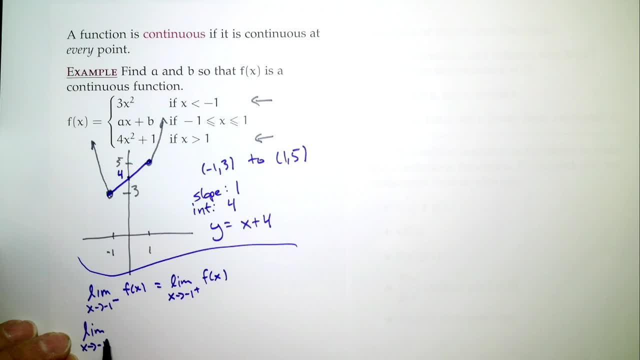 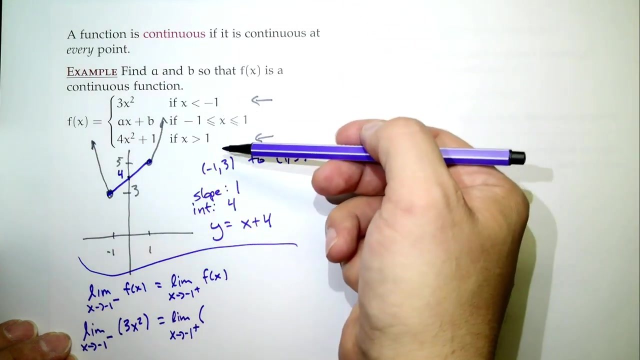 my function is three x squared, So this is limit as x approaches negative one from below of three x squared has to equal the limit as x approaches negative one from above of. and now I go to the part that's just above negative one. I don't want the part that's way above negative one. 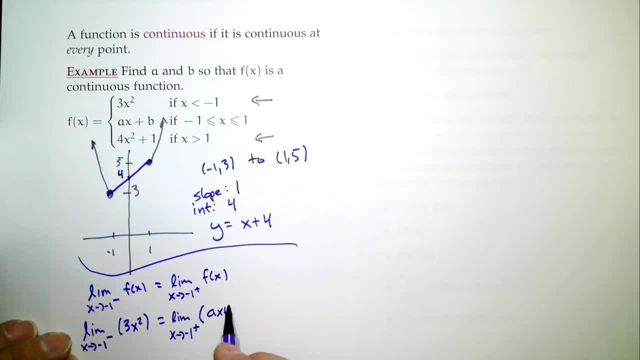 just above negative one. so that's the ax plus b. And now, if we take these limits, because these limits are polynomials, we come to the conclusion that three- which is what happens when I plug in x- equals negative. one has to equal. 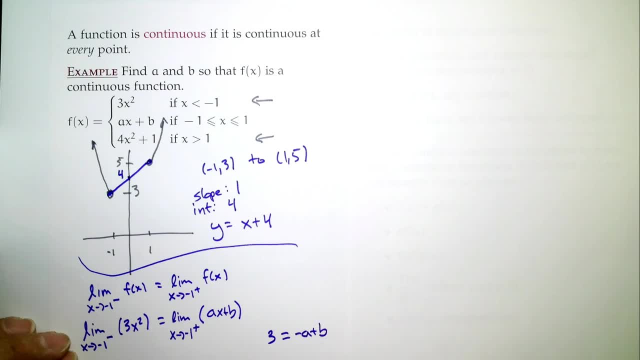 and here it would be negative a plus b, And that's what you would get if you took the limits as x approaches: negative one from both sides. That's half of your setup. The other half is: you repeat this same thing, but now instead. 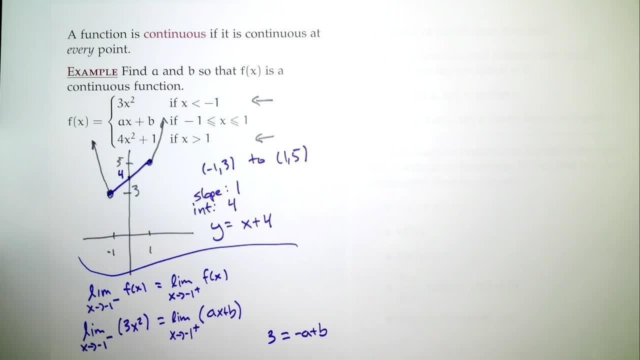 of going limit as x goes to negative one. where do we go? Positive one? So if you repeat that, I'm going to skip the steps. but as limit as x goes to positive one, you're going to end up with five equals. 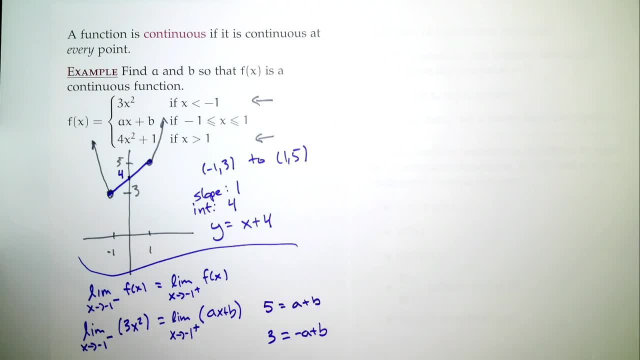 a plus b, And now what you have is you get two equations and two unknowns and off you go. So you don't have to have a picture. The key thing is just to say: I have to make sure these line up. So I've checked. 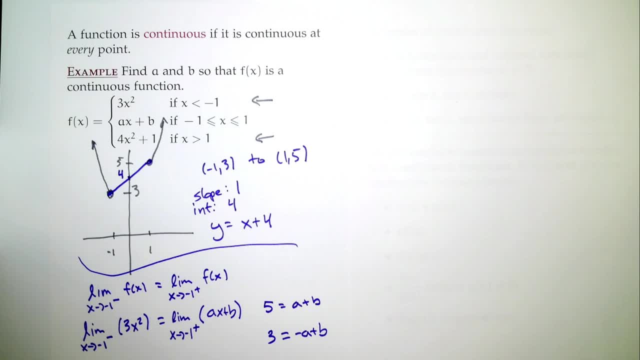 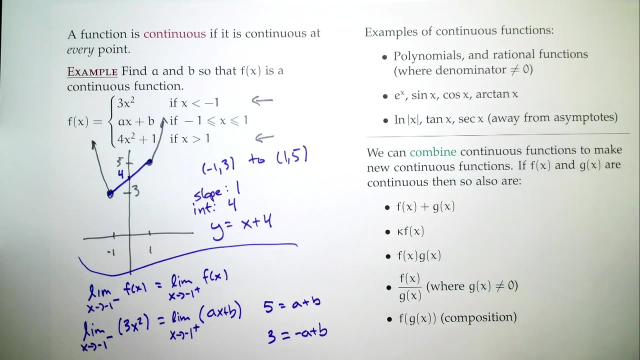 to make sure that the two one-sided limits agree, And for every single potential problem point, in other words, every place where you're gluing parts together, you're going to get an expression. So there you go. Alright. Now what are examples of continuous functions? 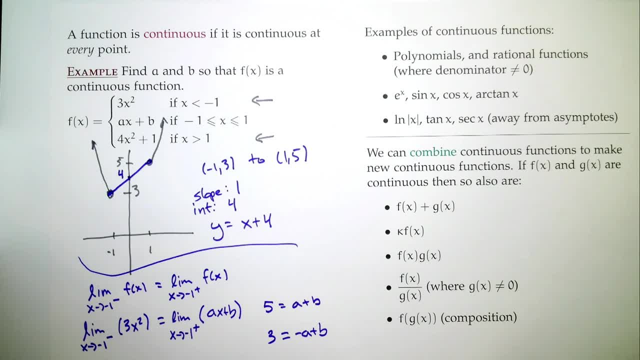 Well, polynomials are, And as well as rational functions, And so a rational function just means a polynomial over a polynomial. You also have other functions: Your e to the x, your sine x, your cosine x, the best function of all, 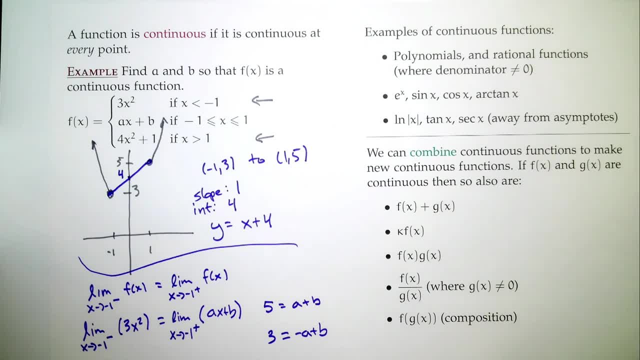 the arctangent of x. It's a really cool function. You also have other things like square root of x. As long as you're talking about x greater than zero, There's a small catch at x equals zero and it's undefined below zero. 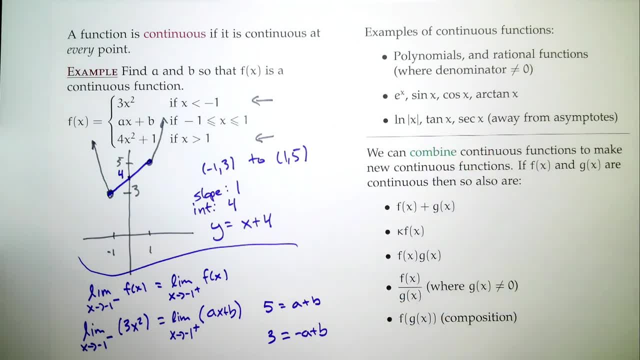 There's some tangent of x and secant of x. These are also continuous as long as you stay away from your asymptotes. So a lot of the functions that we're familiar with are continuous functions, And essentially that's good, because continuous functions are nice. 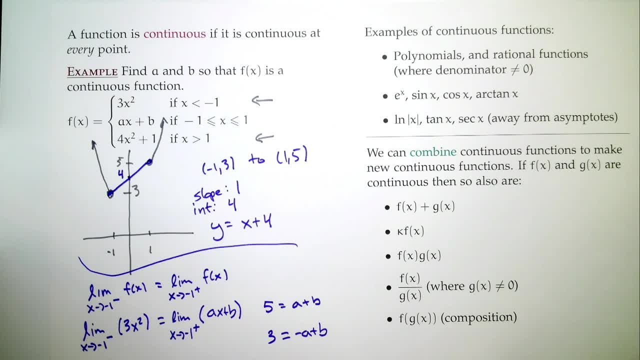 We saw at the very beginning that if we have a small problem with our continuity it can cause weird things to happen. But the other thing are continuous functions make sense to describe phenomenon that we see around us, Because the moral of a continuous function says: if you change a little bit. 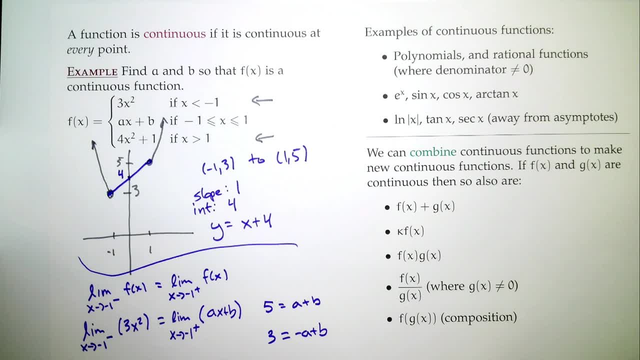 of your input. you can't change your output by a lot, You can't all of a sudden jump a huge amount, And so continuous functions are the right types of functions to model what we see around us Now. the nice thing is, we can combine continuous functions. 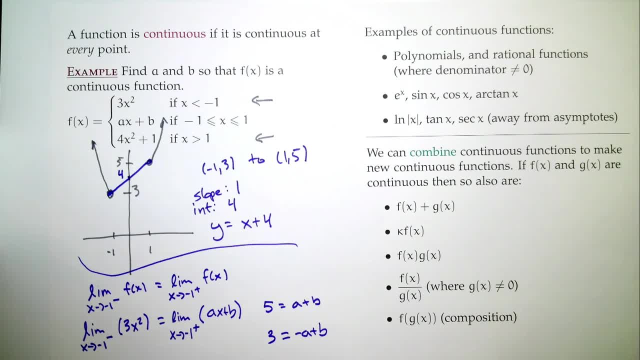 And so if we have a few building blocks, the next thing is: how can we put them together? And these look like the same kind of things we talked about with limits, because that shouldn't be surprising. Continuous functions are really defined in terms of limits. 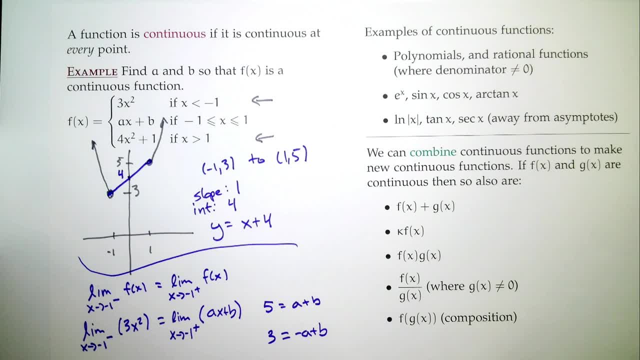 So if you have things which are continuous and you add them, it's still continuous. You can scale continuous functions. That's what's happening here. That's a constant. You can multiply continuous functions, They're still continuous. If you divide a continuous function by a continuous 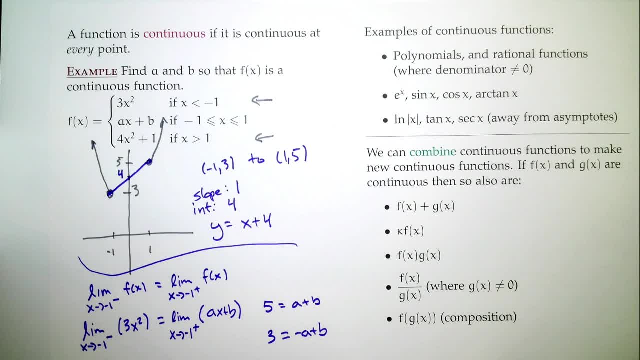 function. as long as your denominator is not zero, you're continuous. The most important one, probably, is composition Function inside of a function. If you have a continuous function inside of a continuous function, you're still a continuous function, Alright. 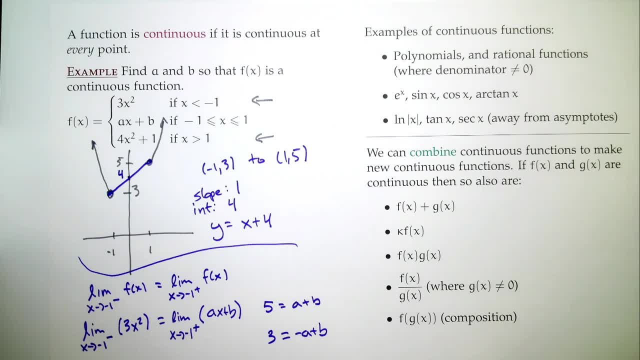 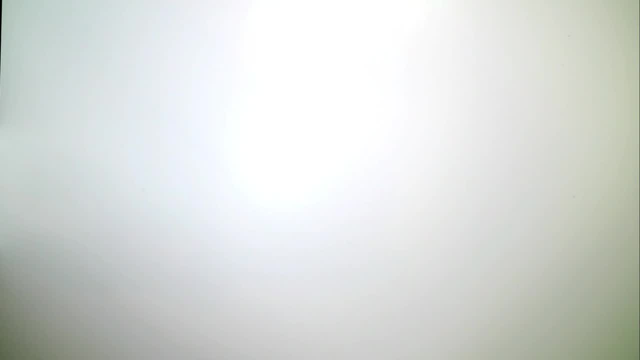 Well, let's try this Alright. So here we go. Is the following function continuous? So sine of e to the x squared plus 23, plus x to the fifth times, arctangent of x minus 17 times cosine of sine. 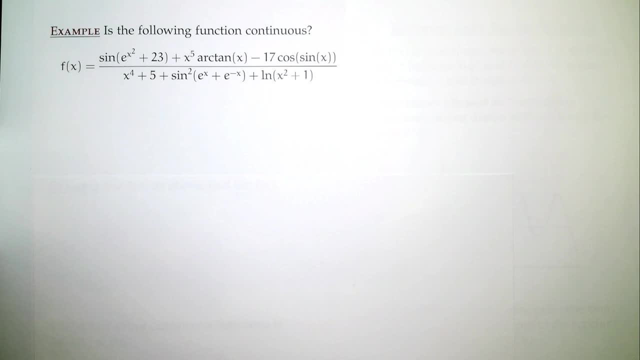 of x. That's the numerator That's divided by x to the fourth plus five, plus sine squared, of the quantity, e to the x plus e to the negative x plus the natural log of x squared plus one. Alright, Good, Now you might think. 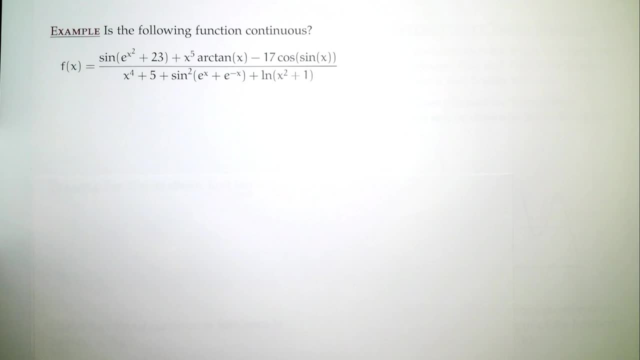 that wasn't on the list. Well, it wasn't quite on the list, but the question is: can we build up to it? So we think about our various pieces. So let's go through the top And let's just start with the term on the left. 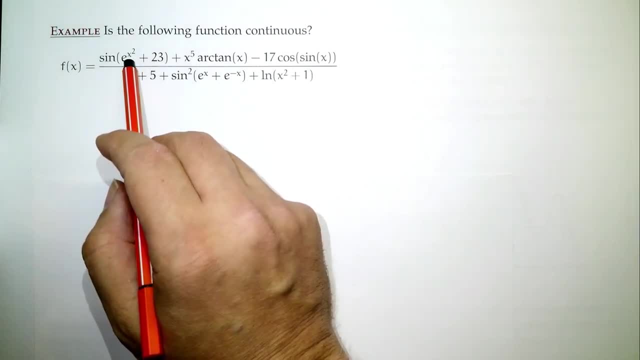 Well, is x squared continuous? Yeah, it's a polynomial. Is e to the x squared continuous? Yeah, Because it's a composition. e to the x squared plus 23?? Yeah, because I adding continuous functions, that's continuous. 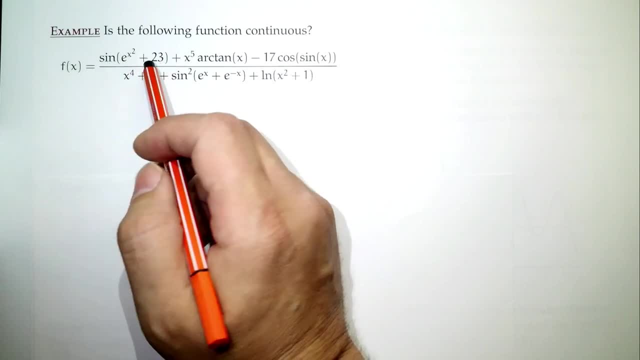 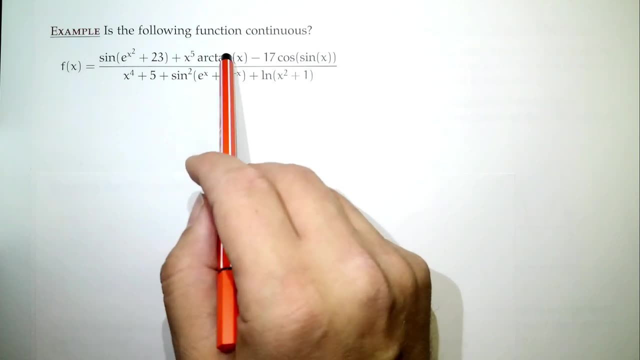 Sine of e to the x squared plus 23? Composition, Composition. Okay, so the first part is continuous. Is x to the fifth continuous? Yeah, polynomial Arctangent of x? Yes, because it's the greatest function of all time. 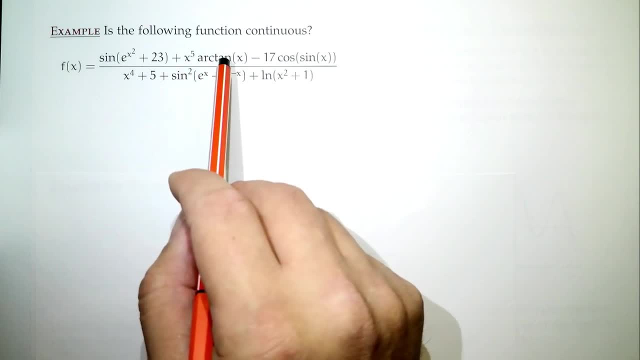 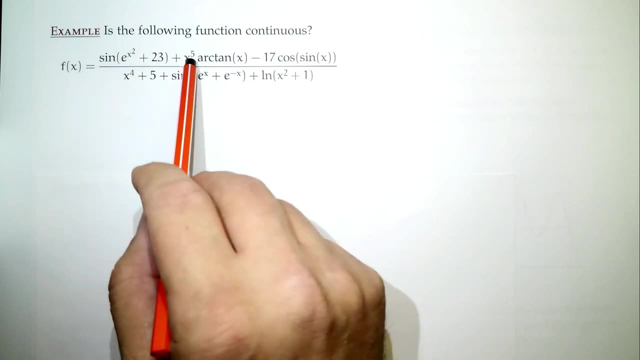 Multiply x to the fifth times arctangent of x. Is that continuous? Yeah, because products of two continuous functions are continuous. So now I have a continuous function plus a continuous function, So still continuous. Alright, sine. is that continuous? 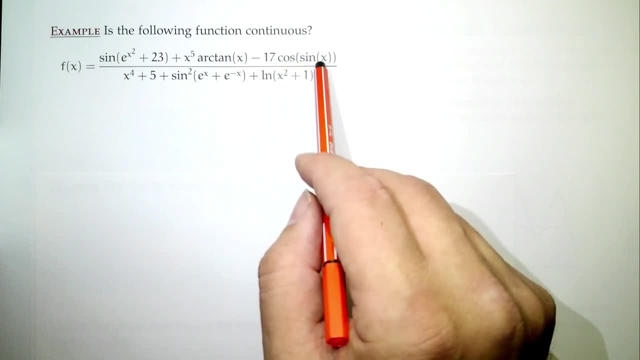 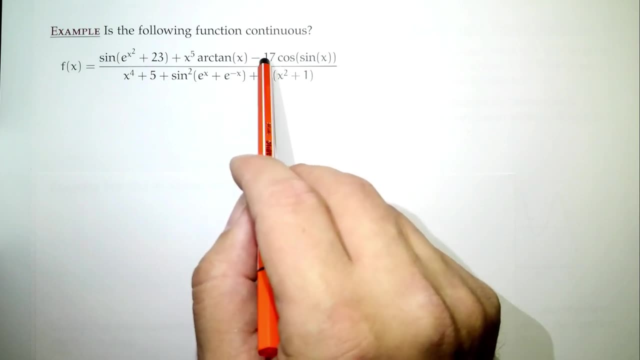 Yes, Is cosine of sine continuous? Yeah, because of composition. If I multiply by 17,, will it still be continuous? Yes, because I can scale by a constant. And then if I combine it with something else, by subtraction, is that still continuous? 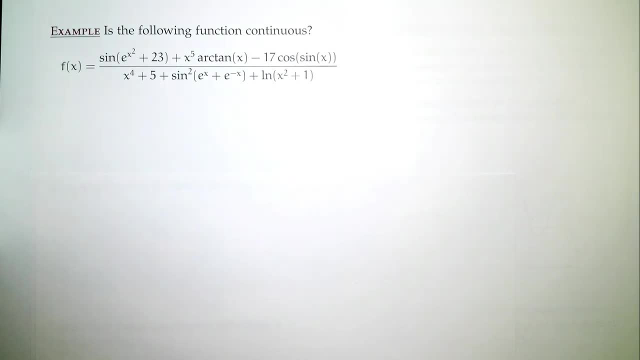 Yeah. so see, we're building up And we don't write all these things down because it would take a long time, but we seem like, yeah, we've got our building blocks Downstairs, Okay. x to the fourth polynomial. Five polynomial: 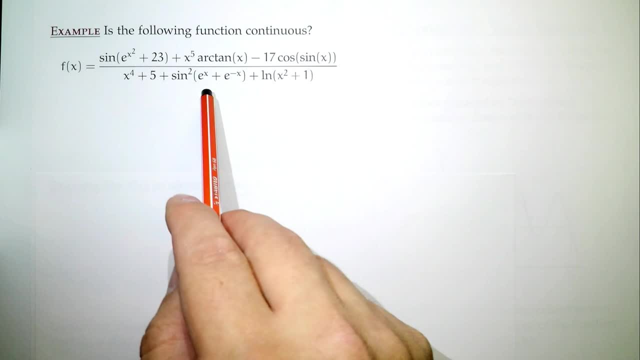 e to the x plus e to the negative x. is that continuous? Yeah, We have a composition and we have adding two continuous functions. Then it's plugged into sine squared. is that continuous? Yeah, because we first plug it into sine. 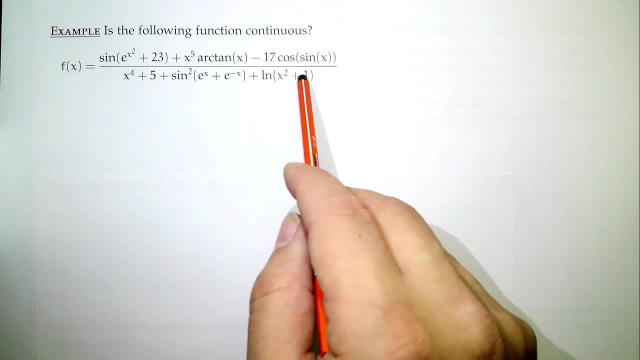 which is continuous. then we square it, which is continuous, x squared plus one polynomial continuous Log of x squared plus one composition. We add them all together. is it downstairs continuous? Yeah, Now, as long as. yeah. someone said: as long as. 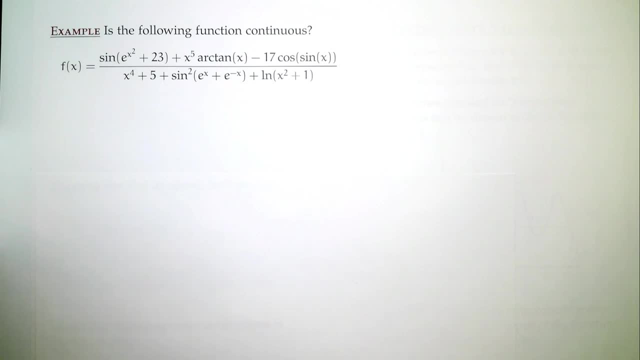 it's not zero, Alright, Can the downstairs ever be zero? Well, now we're kind of paranoid. We've been hurt before, Alright? Well, certainly notice the x to the fourth. That can't be negative. Sine squared can't be negative. 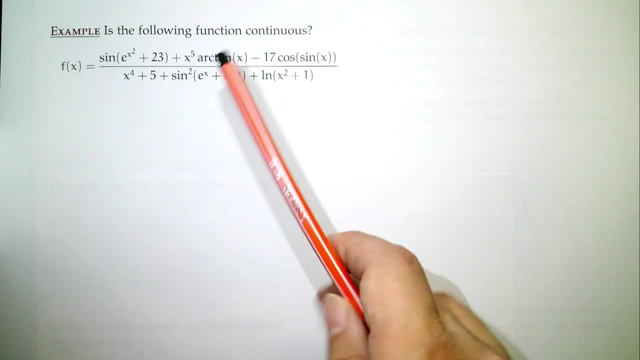 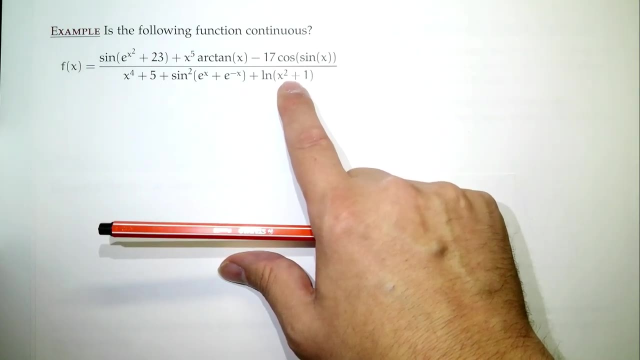 What about log? Log could be negative, but look at the inside of the log. How small can x squared plus one be One? That's the smallest they can get, What's the well? okay, so log of one is zero. 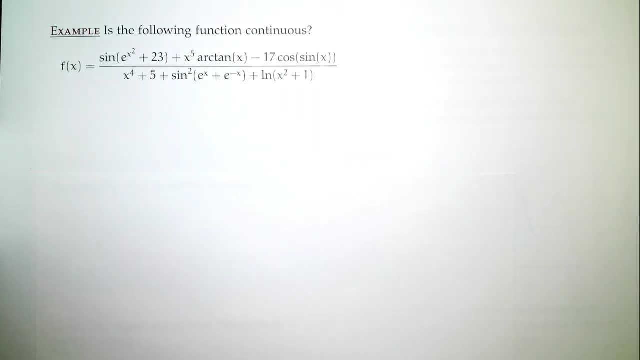 And if you plug anything bigger than one into log it's positive. So all the three terms there are all at least zero, and then you have a plus five. So that definitely bumps you away from zero. So this function is continuous for all values of x. 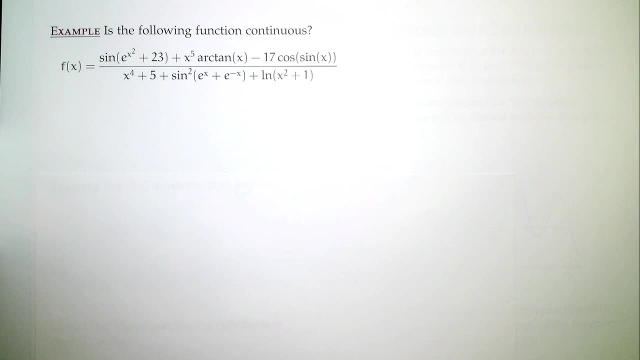 no problems. Cool. So the answer is yes, Alright. Well, in case you're wondering, is there ever going to be an exam problem where you just have to write down the word yes, No, No, Well, sometimes there's multiple choice. but 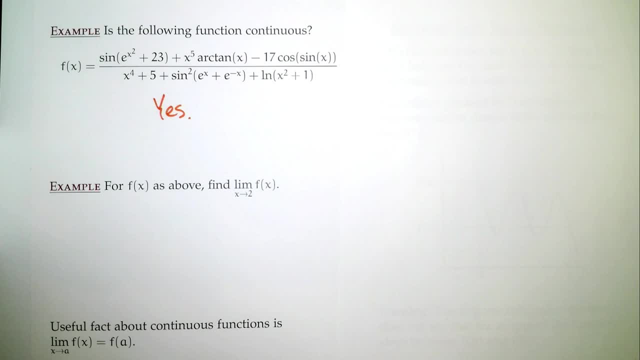 you never want the multiple choice. Oh, I should hide that. Pretend like you didn't see that. Alright, So suppose I have f of x as above. So there's my function, f of x, and I want to find the limit. 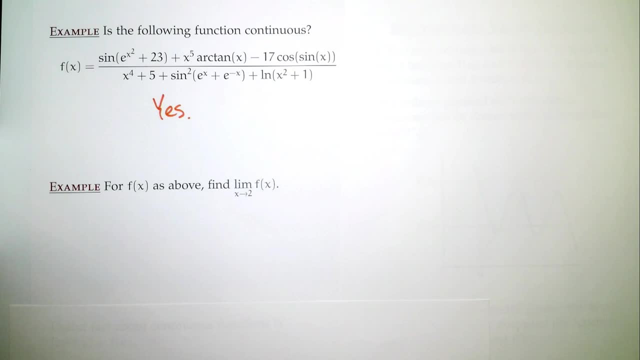 as x approaches two of f of x, You're probably thinking that sounds like a much harder limit than all the ones that we've done so far, Or is it? Is there an easy way for us to do this limit? Plug it in. 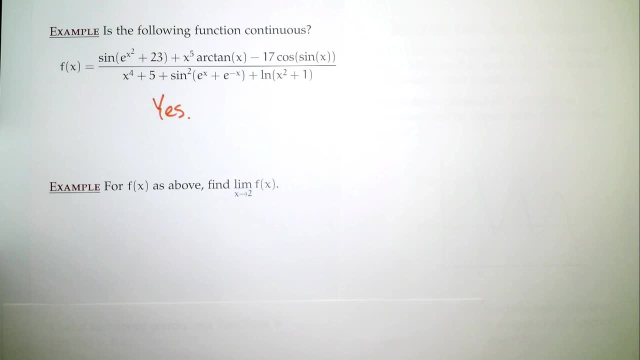 Why can we just plug it in? Because it's continuous. See, continuous things have this beautiful property: A function that's continuous. if I want to know what the limit is, I just plug in the value And therefore the answer is: 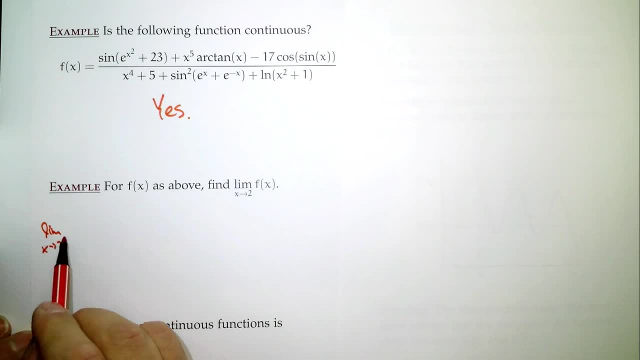 the limit as x approaches, two of f of x. This is not a hard thing, it just takes us a long time to write down. It would be sine of, I guess, e to the fourth plus twenty-three two to the fifth, which of course we all know that's equal to. 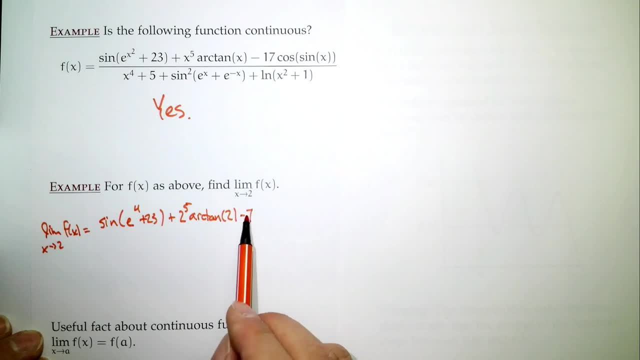 thirty-two, arc tangent of two minus seventeen, cosine of sine of two divided by two to the fourth, which is sixteen. but we can write it as two to the fourth plus five plus sine, squared e, squared plus e to the negative, two plus log of two squared. 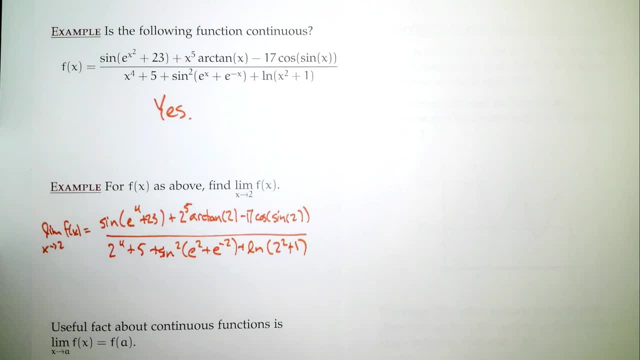 plus one, And that's it, we're done So. you always like continuous functions. Continuous functions are your friends. If you have a continuous function, you always sort of say, hey, if I'm taking the limit of something that's continuous, the 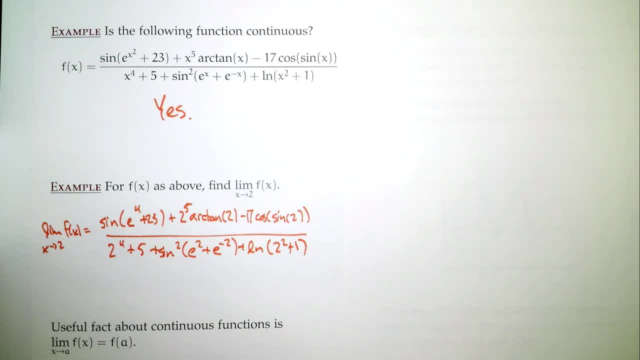 first thing we should always do is just plug it in, Because maybe whoever wrote the problem wasn't paying attention, Or maybe they're trying to make sure you're paying attention and not trying to do something. that's too hard, Alright, So. 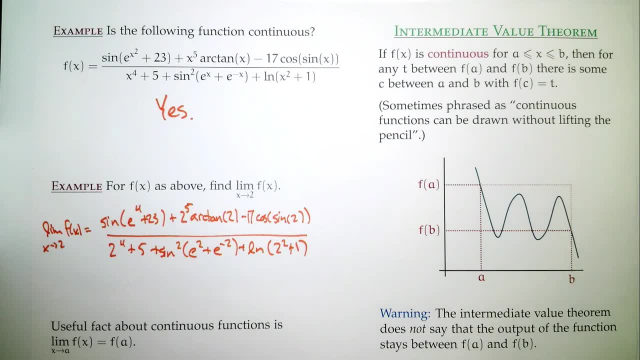 we need another one more important idea today and some examples. There's something called the intermediate value theorem And it deals with continuous functions. It says, suppose I have a function which is continuous, So I have a continuous function, and it's continuous, say starting at a. 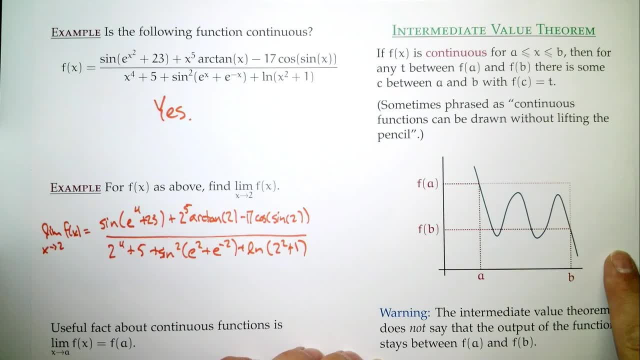 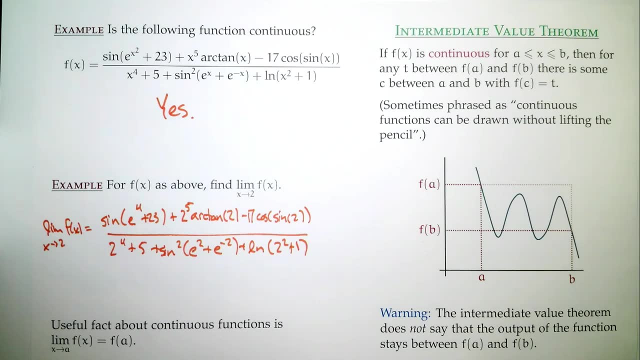 and going to b. What happens above b and what happens below a, we don't care, But between a and b it's continuous. Then what has to be the case is that where I start. so I start at this value here: f of a. 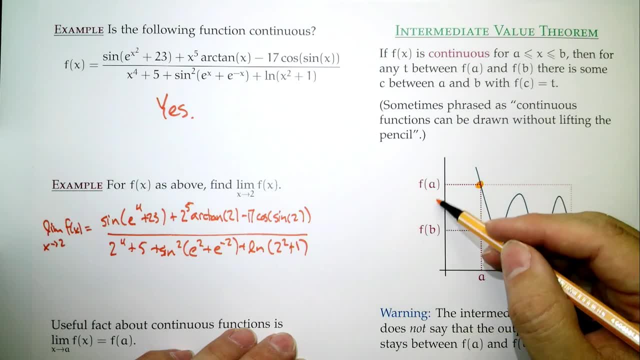 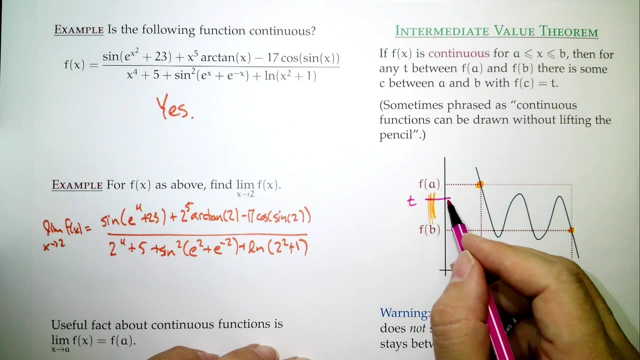 and where I stop is value f of b. So there might be some space here between f of a and f of b And if I pick anything that goes between f of a and f of b, so suppose I pick this is my value here t. 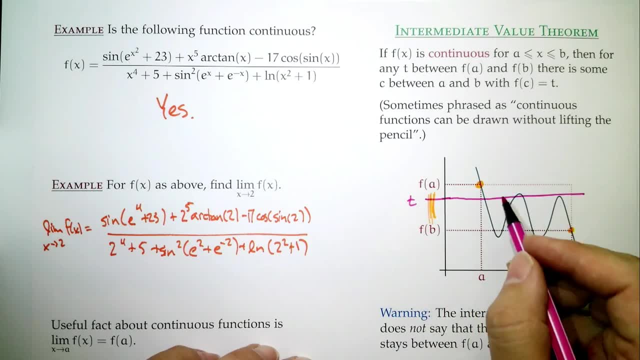 and I were to draw this line straight across. what has to be the case is: I have to cross it at some point. So at least once It's possible, I cross it multiple times. So it's not saying I only cross once, but it's saying that for any. 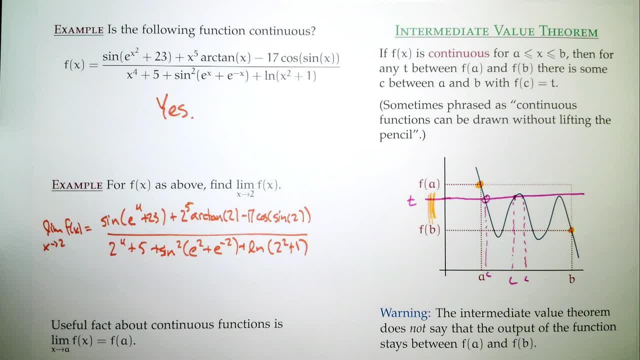 value between f of a and f of b I have to cross through Alright. Well, seems pretty intuitive. It sort of comes back to that philosophy which you may have heard about continuous functions, is you can't lift your pencil up. In other words, if I'm starting at a, 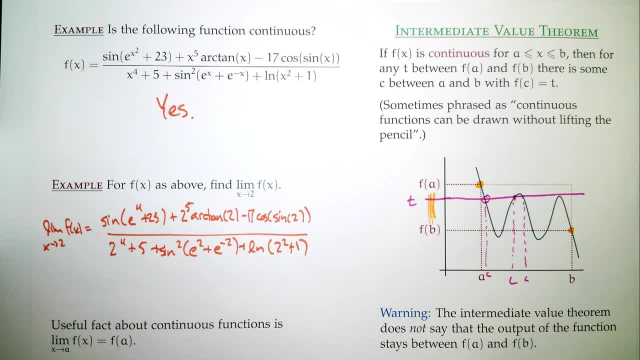 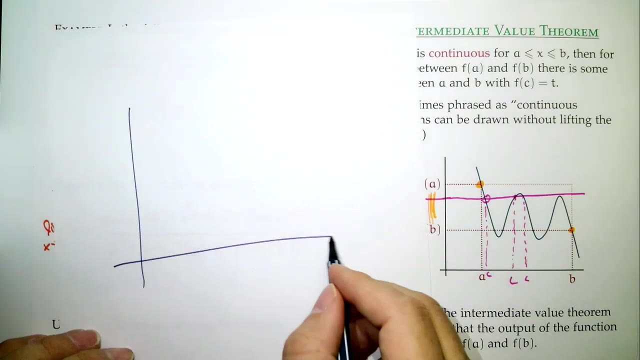 f of a and I keep drawing. I have to cross over everything eventually. Now you might say you know I could get across. Let's see How could we do that. Well, hmm, Maybe I'm not a great artist, but let's say, here is. 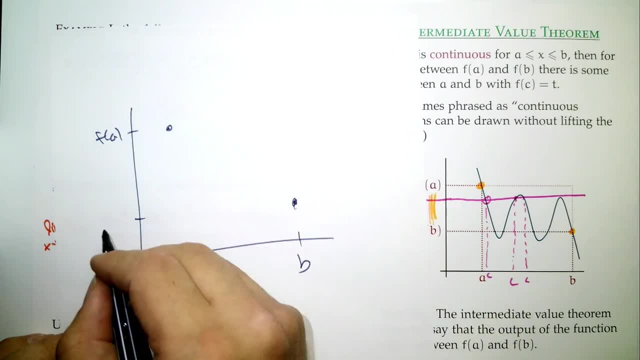 f of a and here is f of b, And we don't make any assumptions, by the way. It could be that f of a is smaller than f of b, or it could be the way that it's drawn here, And you might say: well, 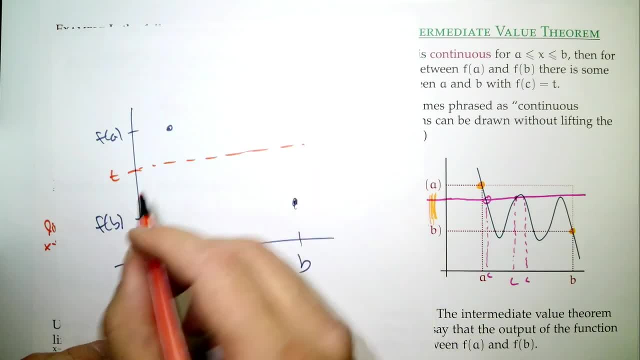 how do I get from this point to that point without lifting my pencil? Well, hmm, The answer, well is, channel your inner Mario Brothers, Look for the pipe right. And so that way it's really easy. You just say: 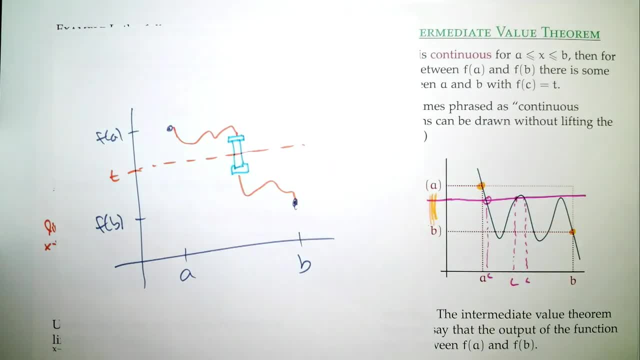 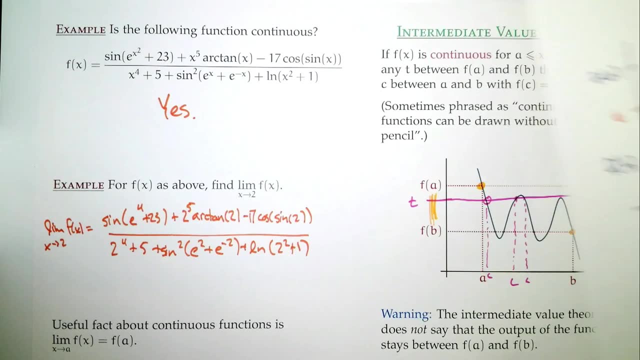 mm-hmm, doo-doo-doo, whoop, But okay, No, no, There is no pipe. Pipes don't exist in our world, So you cannot avoid it. You have to cross through the points, So uh. 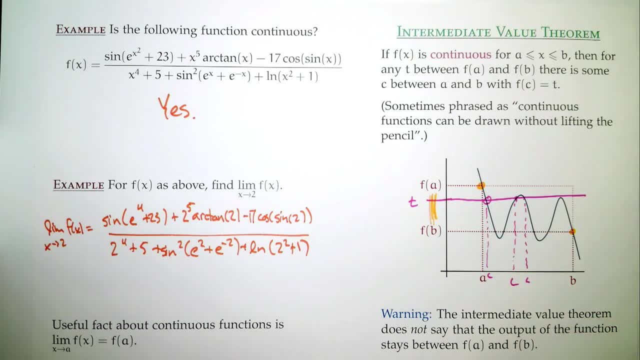 just in case I haven't said it. let me point out this warning because there tends to be the when you hear the statement of the Intermediate Value Theorem. the Intermediate Value Theorem says: I have to hit all the values in between. 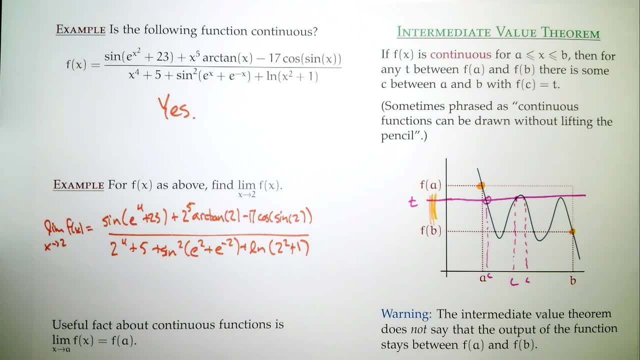 Sometimes people hear that and say: oh, that means that you're going to stay in between, And that's not what the Intermediate Value Theorem says. So it's possible that you can sort of sneak your way below at some points You'll notice. for instance, there's a few times 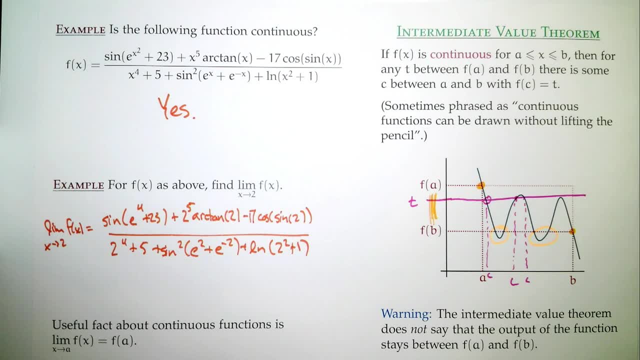 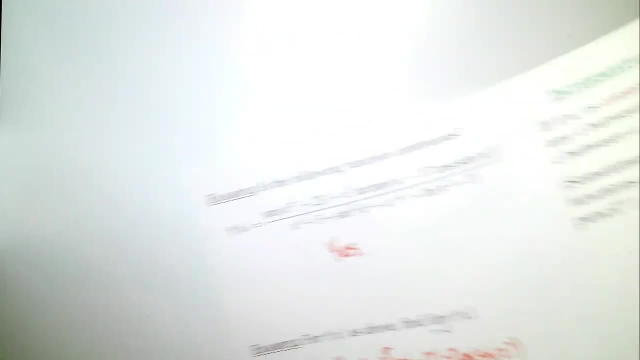 when the curve dips outside of that interval between f of a and f of b, and that's okay. The only thing we can say for sure is that everything in between it got some point where I got the evaluation Alright. Well, let's. 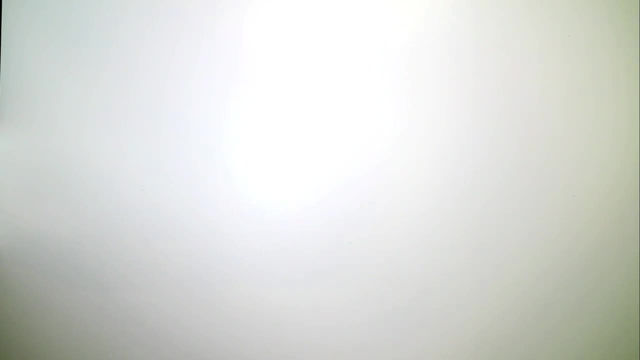 test our intuition, Here we go. Here's a polynomial: 18x cubed minus 63x, squared plus 67x minus 20.. And there's two questions here. So part a, Does f of x have a root in the interval between 0 and 1?? 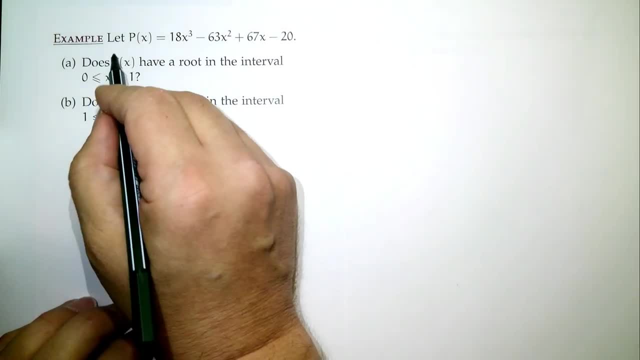 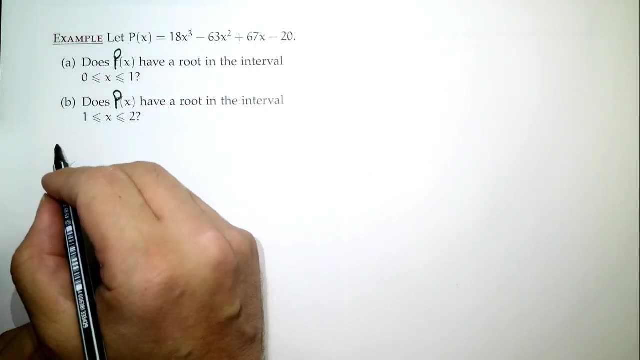 And there's another typo. This should be p. Alright, sorry about that, I'll fix that later. So does this polynomial have a root in the interval 0 to 1?? So what do we mean by root? So a root means there's some number. 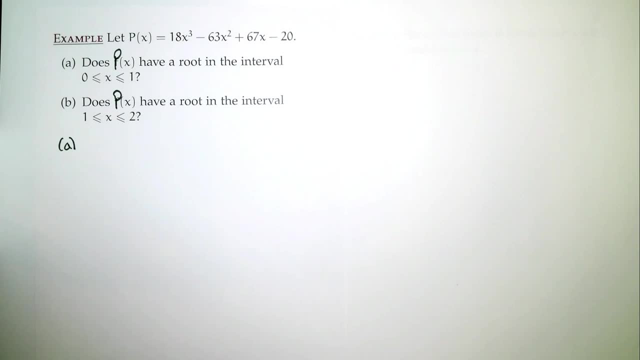 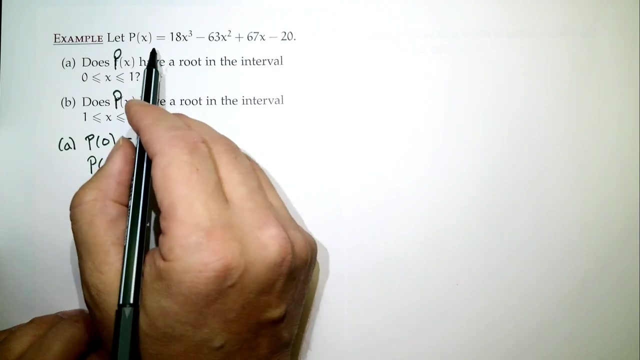 which I can plug in and I get 0 out. That's what a root means. So, channeling what we just learned, let's look at the values p of 0 and p of 1.. What do I get when I plug 0 in? 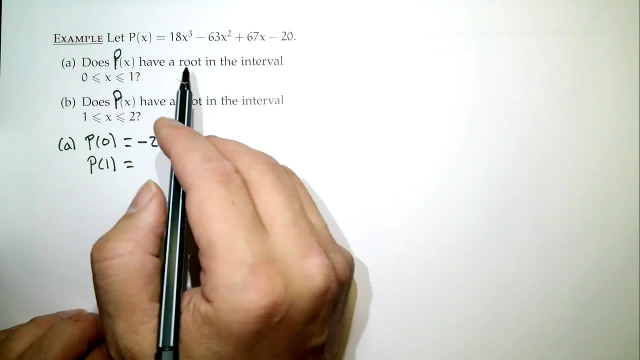 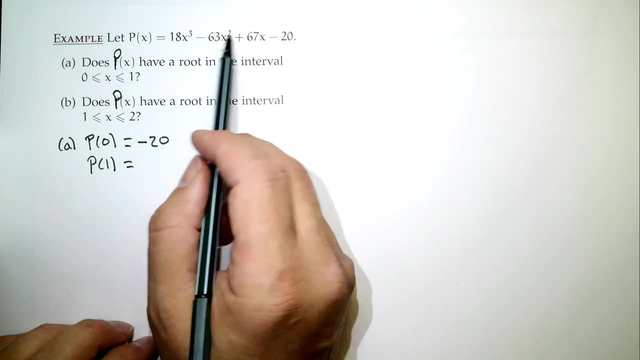 Negative 20.. How about when we plug 1?? That one's probably not quite so fast. What do you see? Well, you see an 18 and a 67. Those will combine together to give you 85. Then you see a negative 63 and a negative. 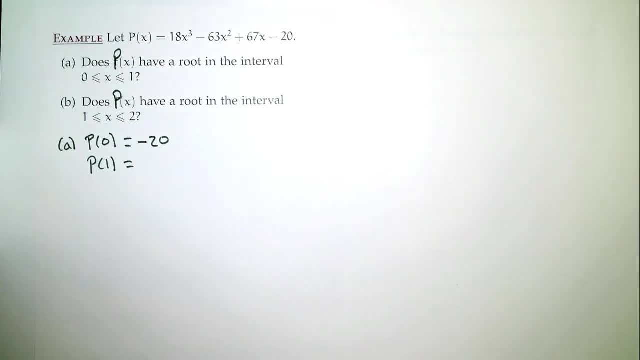 20.. Those will combine together to give you negative 83. So you end up with 2.. Now what does this say? This says: at 0 you're negative, at 1 you're positive. So what has to happen somewhere in between 0 and 1?? 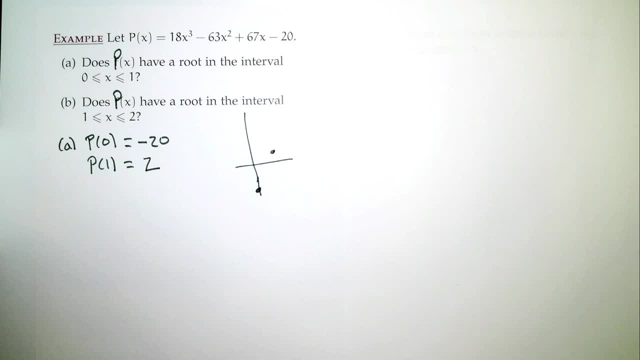 Yeah, you have to pass through that 0. It has to be a root. So intermediate value theorem says there's a root. Now we should be careful. We know that there's at least one. Could be more than one. 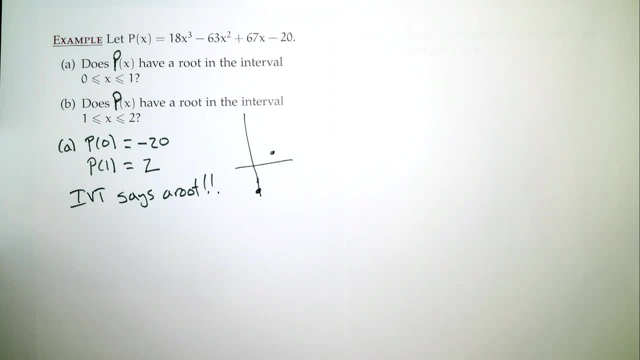 but there's at least one. So if you ever switch from positive to negative, then you have to have a root. Well, actually we forgot to say something. What else do we have to check before we apply the immediate value theorem? Is it continuous? 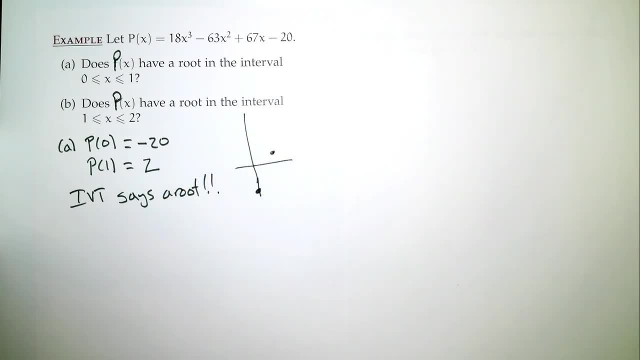 Yeah, we didn't check that. Is this function continuous? Yeah, it's polynomial. Good, Okay, But we want to make sure, we want to dot all our i's cross, all our t's, Alright. So that's part A. Part B. 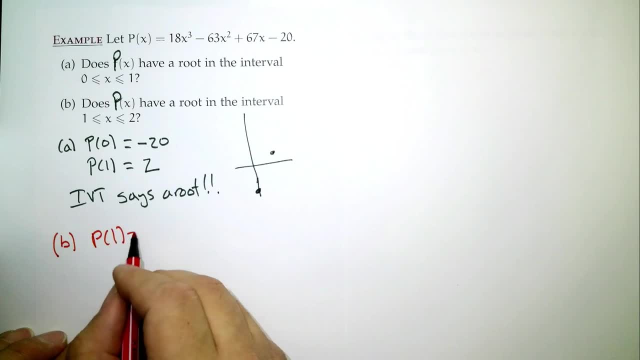 How about between 1 and 2?? Alright, 1. Well, we know what happens when we evaluate at 1. We got 2, because I'm just going to copy my work. 2. Well, hmm, Huh, What is that? Well, it's. 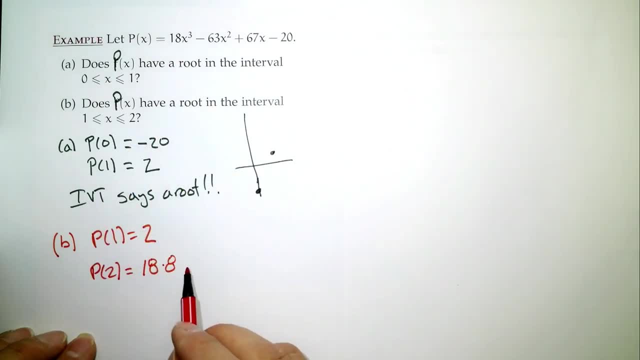 18 times 2, cubed, which is 8, minus 63 times 2, squared, which is 4, plus 67 times 2, minus 20.. 18 times 8 is, of course, 144.. That's right, Yeah, Cool. 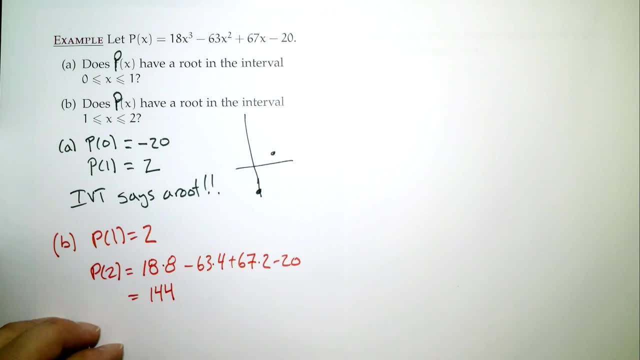 You knew it. I was wondering if anyone was going to say gross. I was like, yeah, that's also right, Alright, But anyways, 63 times 4 is 252.. 67 times 2 is 134.. And 20 is 20.. 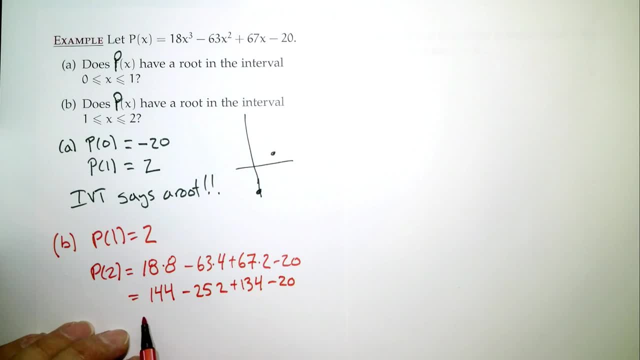 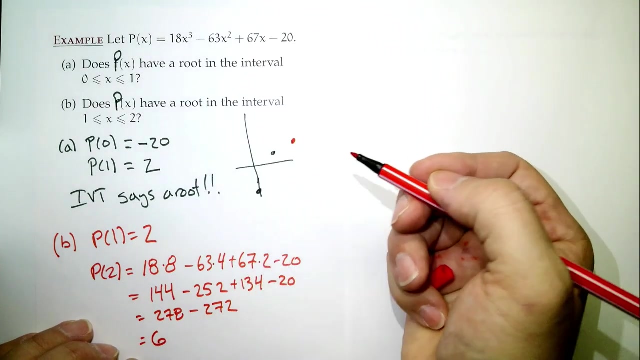 So 144 plus 134.. That's 278.. Then we're going to subtract off 252 and 20.. That's subtracting off 272, giving us a grand total of 6.. Which means we are over there. So at 1, we're at 2.. 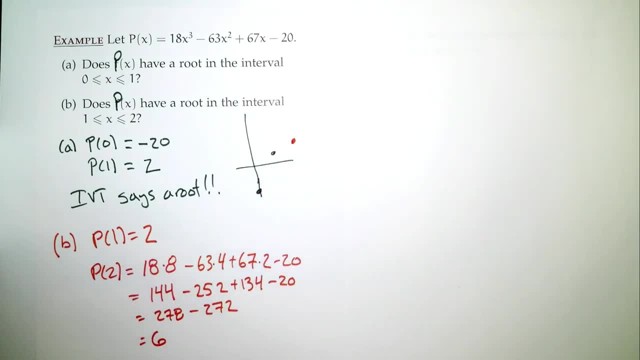 And at 2, we're at 6.. So is there a root between 1 and 2?? Our answer is: We have no idea. Now you're probably thinking: wait a second. We start positive, we end positive. 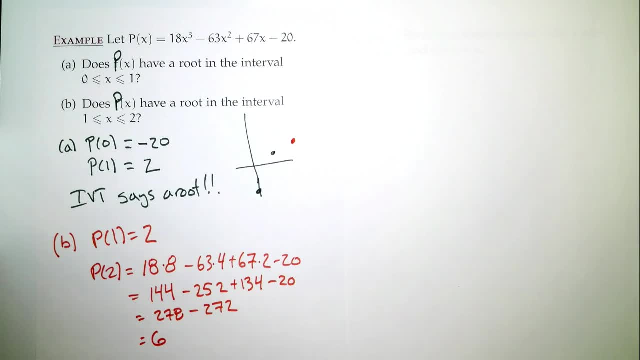 there's no root. But remember what we said. Be careful about what the Intermediate Value Theorem says. It doesn't say that you have to stay between them. It just says you have to hit everything in between. What could potentially happen is that you could. 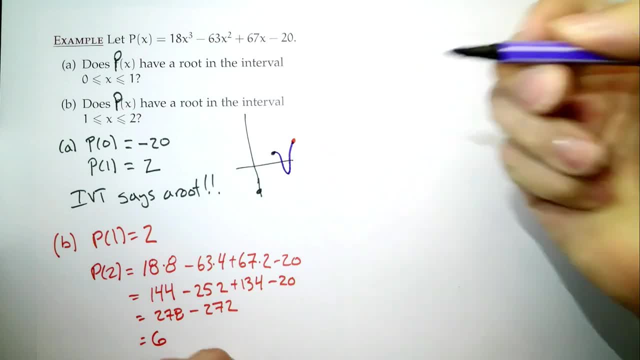 actually dip down and come back up. Now I say: what potentially could happen is that? you see that, because it actually does happen- It turns out there are two roots between 1 and 2.. So be careful: Just because you stay the same sign doesn't mean that. 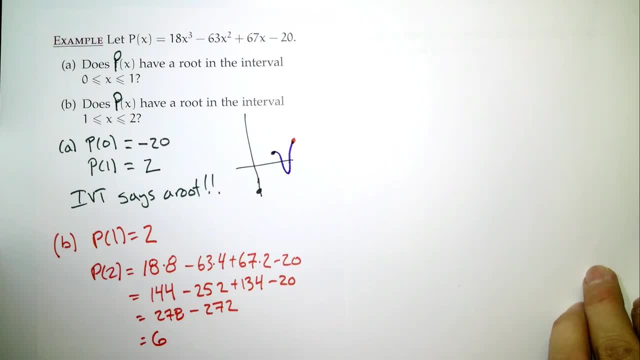 you had a sort of a brief fling with the negative side. Alright, I think we've got enough time to talk about this last part. Show that there is some value x between 0 and 1 where cosine of x is equal to x. 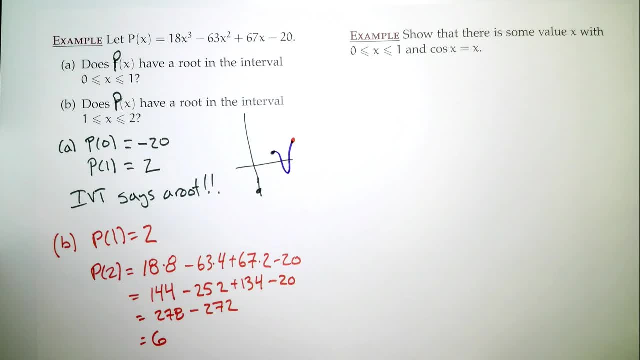 I don't know if you ever did this: when you have a calculator, one of those old scientific calculators, and you would just like push the cosine button and you'd update and like, oh okay, let me push it again. And then you're like, let me keep. 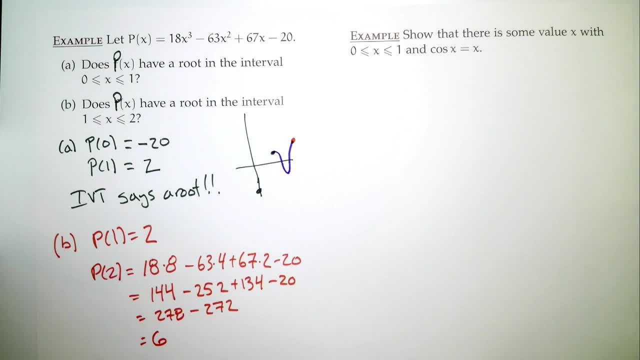 pushing it. And if you do that, what happened? eventually? You didn't get an error, Unless you pushed really hard. Well, what happened is that you'd start getting to a very particular number. Alright. Now how could you argue this? 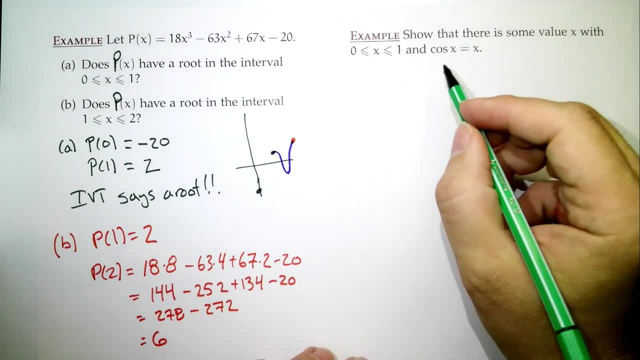 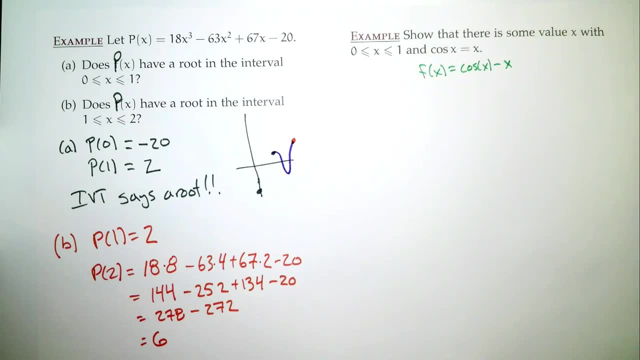 Well, there's a couple ways to do this. You could say I can think of this as f of x. Let me look at cosine of x minus x. If we're looking at it in that way, what are you looking for? 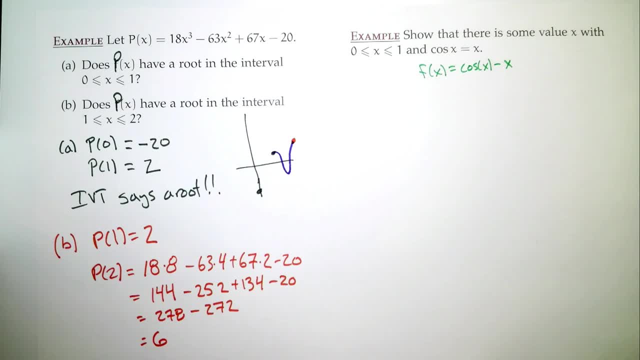 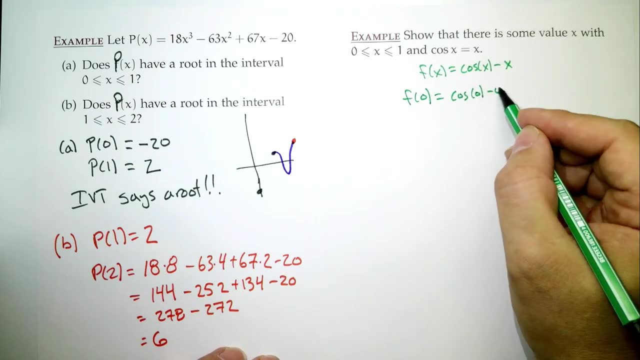 You're looking for a root, So I just have to argue that there is a root. Let's think about what f of 0 is. Well, that's cosine of 0 minus 0, which is 1.. That's a positive number. 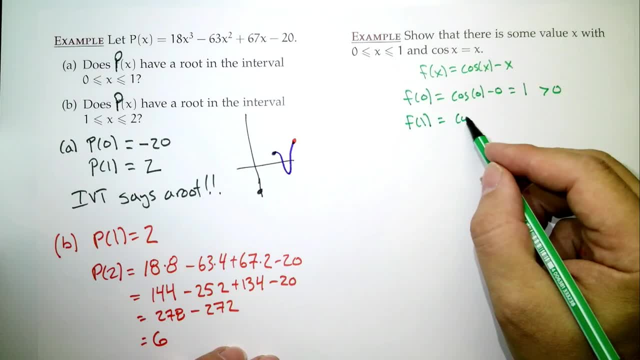 What's f of 1?? Well, that's cosine of 1 minus 1.. Now, I don't know the exact value of cosine 1, but I do know something: It's not 1.. In fact, it has to be less than 1.. 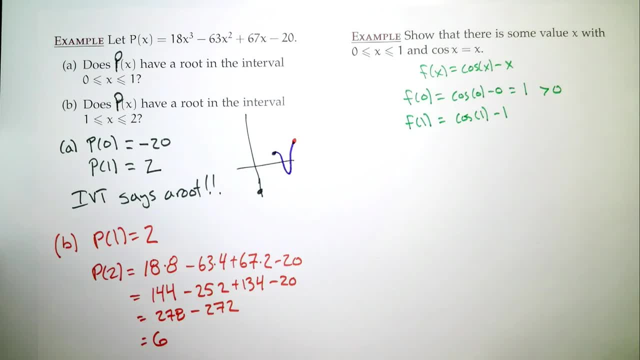 So cosine of 1 minus 1, what kind of number is it? It's negative. So if I start out positive and if I end up negative, what has to be the case? It has to be a root. So this is enough. 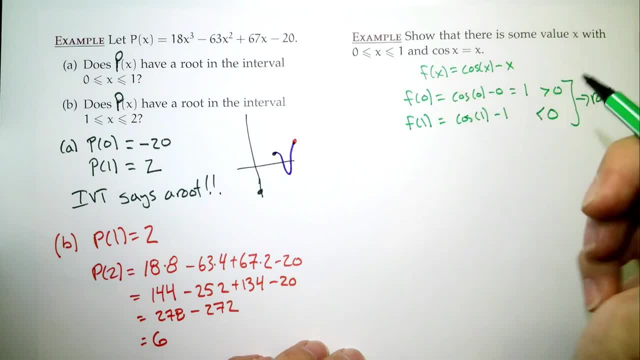 to say there has to be a root between 0 and 1.. Of course we should have also pointed out what is true about f of x: It's continuous, But here's sort of a different way to think about it, And this is fun. 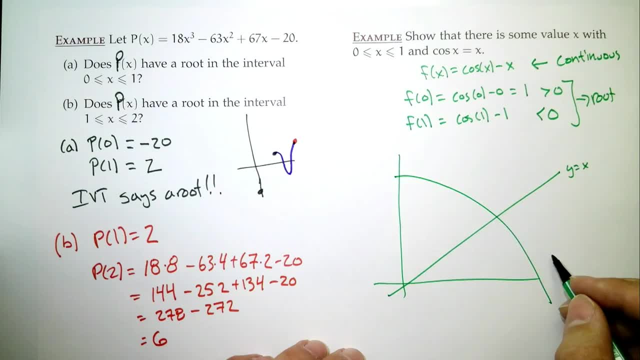 So start with y equals x, Start with cosine x And here's what you can do. This is what's happening when you do your calculator. When you first plug in, start at 0,, plug in your cosine, you say, aha, that goes.